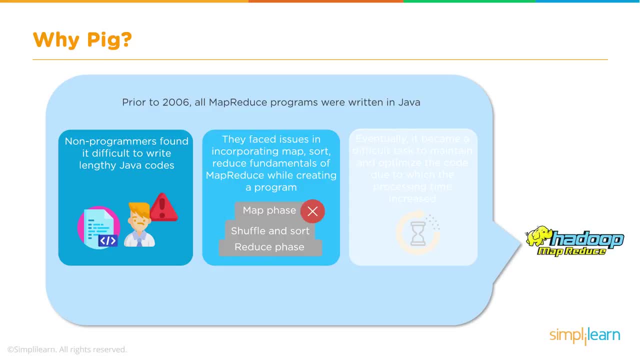 They faced issues in incorporating MapReduce, So they had to map, sort, reduce to fundamentals of MapReduce while creating a program. You can see here: Map Phase, Shuffle and Sort Reduce Phase. Eventually, it became a difficult task to maintain and optimize a code, due to which the processing time increased. 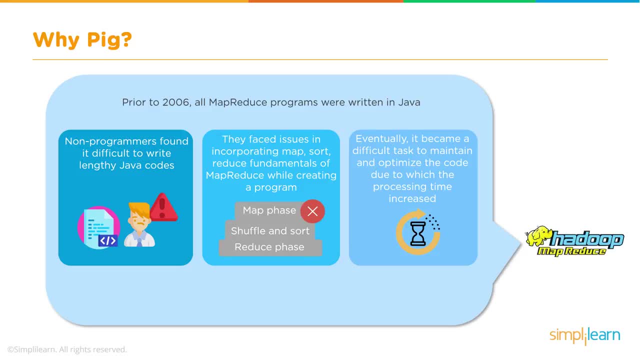 You can imagine a manager trying to go in there and editing a simple query to find out data and he has to go talk to the programmers anytime he wants anything. So that was a big problem. Not everybody wants to have an on-call programmer for every manager on their team. 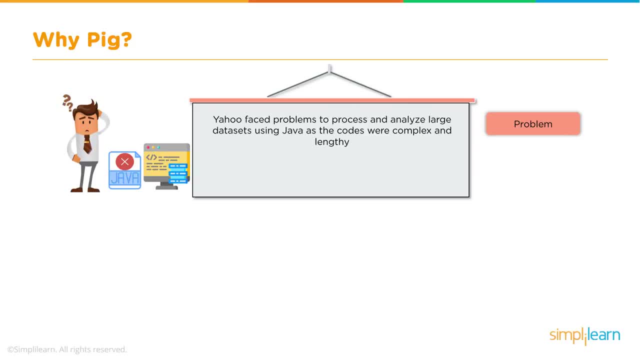 Yahoo faced problems with MapReduce. They had problems to process and analyze large datasets using Java, as the codes were complex and lengthy. There was a necessity to develop an easier way to analyze large datasets without using time-consuming complex Java modes And codes and scripts and all that fun stuff. 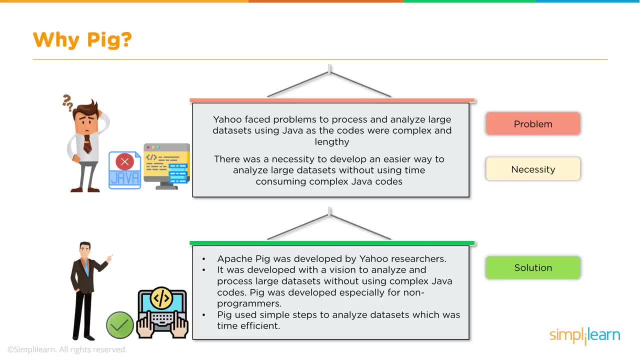 Apache Pig was developed by Yahoo. It was developed with the vision to analyze and process large datasets without using complex Java codes. Pig was developed especially for non-programmers. Pig used simple steps to analyze datasets, which was time efficient. So what exactly is Pig? 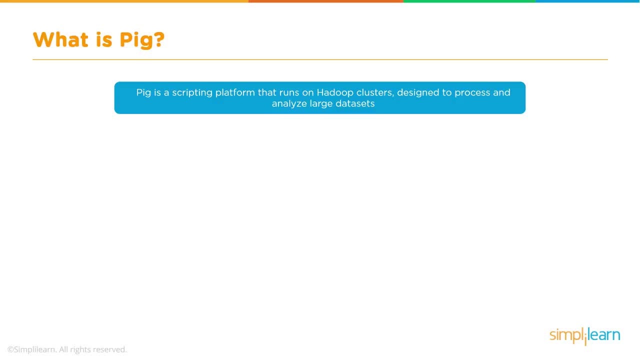 Pig is a scripting platform that runs on Hadoop clusters, designed to process and analyze large datasets. And so you have your Pig, which uses SQL-like queries- They're definitely not SQL, but some of them resemble SQL queries- And then we use that to analyze our data. 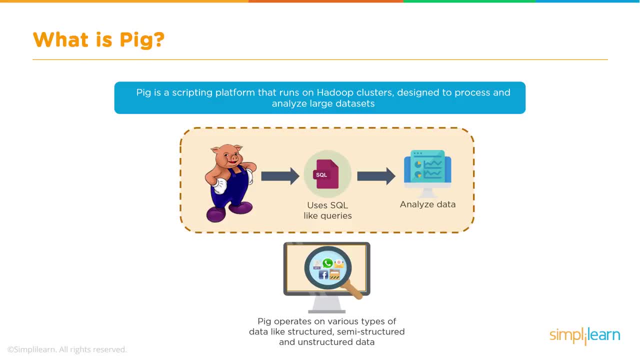 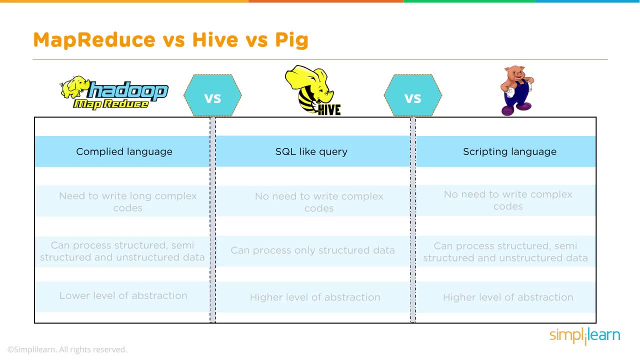 Pig operates on various types of data, like structured, semi-structured and unstructured data. Let's take a closer look at MapReduce versus Hive versus Pig. So we start with a compiled language, your MapReduce, And we have Hive, which is your SQL-like query. 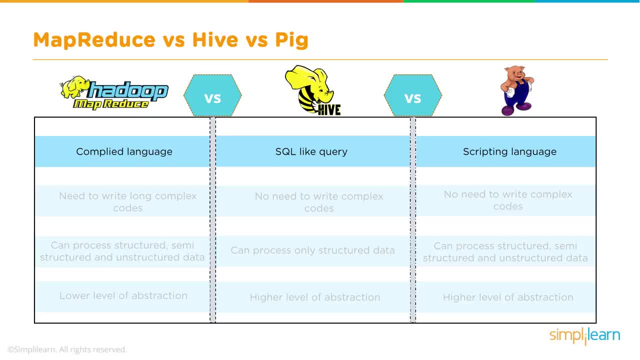 And then we have Pig, which is a scripting language. It has some similarities to SQL, but it has a lot of its own stuff. Remember, SQL-like query, which is what Hive is based off, looks for structured data, And so when we get into scripting languages like Pig now, we're dealing more with semi-structured and even unstructured data. 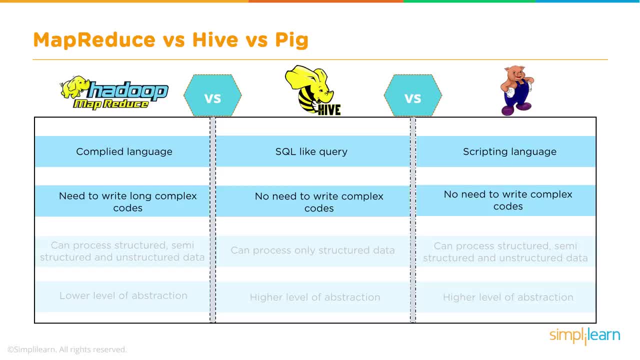 With a Hadoop MapReduce, we have a need to write long, complex codes. With Hive, no need to write complex codes. You could just put it in a simple SQL query or HQL, HiveQL And in Pig, no need to write complex codes as we have Pig Latin. 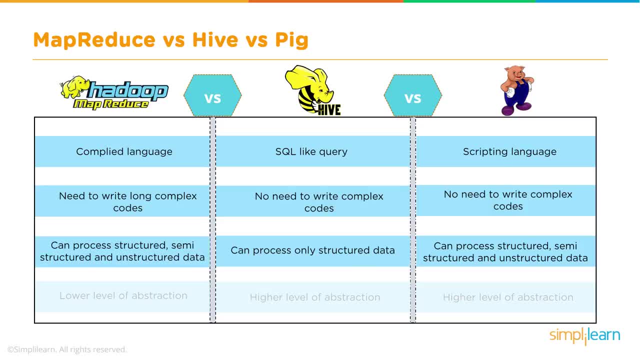 Now remember, in the MapReduce it can produce structured, semi-structured and unstructured data And, as I mentioned before, Hive can process only structured data. Think rows and columns, Where Pig can process structured, semi-structured and unstructured data. 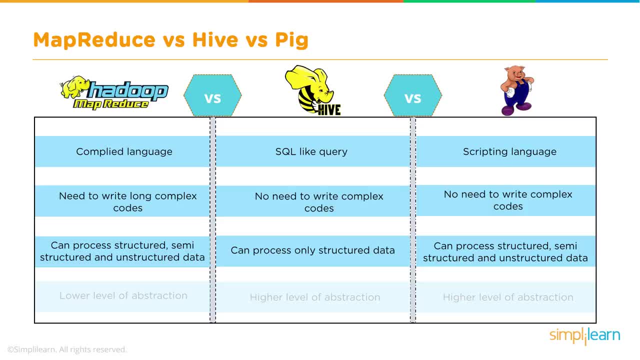 You can think of structured data as rows and columns, Semi-structured as your HTML, XML, XML documents that you have on your web pages, And unstructured could be anything from groups of documents in written format, Twitter tweets. Any of those things come in as very unstructured data. 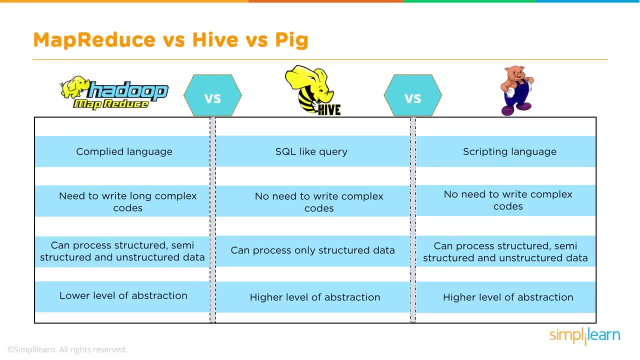 And with our Hadoop MapReduce we have a lower level of abstraction. With both Hive and Pig we have a higher level of abstraction, So it's much more easy for someone to use without having to dive in deep and write a very lengthy MapReduce code. 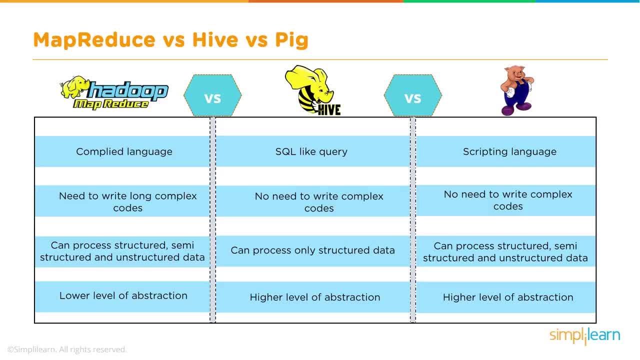 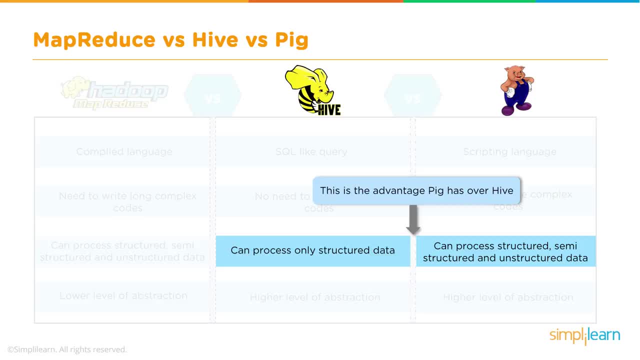 And those Map and Reduce codes can take 70, 80 lines of code When you can do the same thing in one or two lines with Hive or Pig. This is the advantage Pig has over Hive: It can process only structured data in Hive. 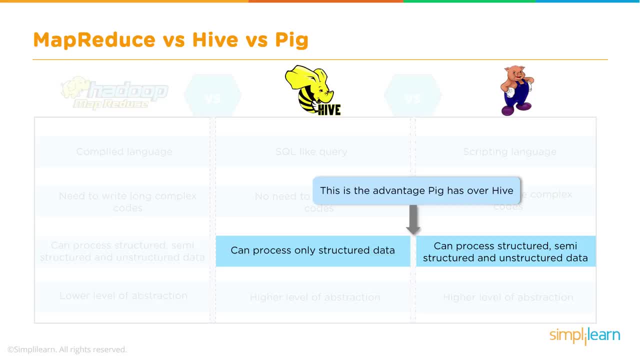 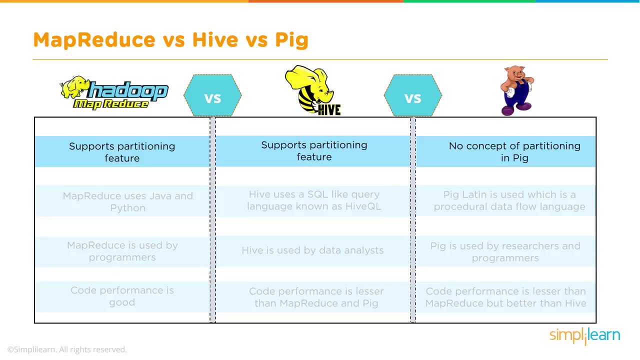 While in Pig it can process structured, semi-structured and unstructured data. Some other features to note: that separates the different query languages. As we look at Map and Reduce: MapReduce supports partitioning features, as does Hive Pig. no concept of partitioning in Pig. 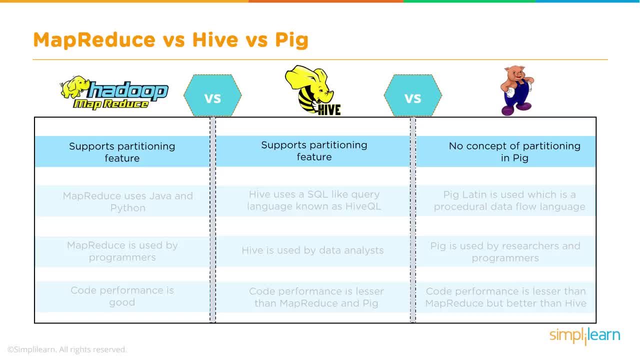 So it doesn't support your partitioning feature. Your partitioning features allow you to partition the data in such a way that it can be queried quicker. You're not able to do that in Pig. MapReduce uses Java and Python, While Hive uses an SQL-like query language known as HiveQL or HQL. 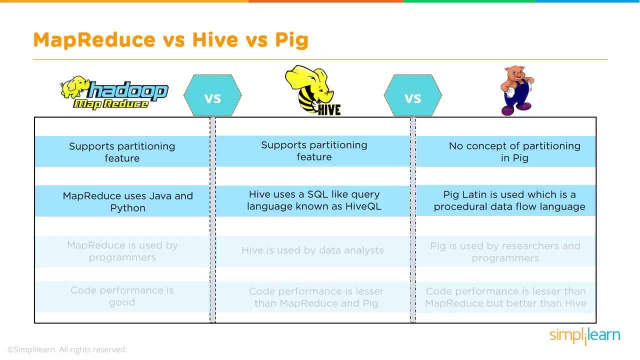 Pig, Latin is used, which is a procedural data flow language. MapReduce is used by programmers. Pretty much is straightforward on Java. Hive is used by data analysts. Pig is used by researchers and programmers. Certainly there's a lot of mix between all three. 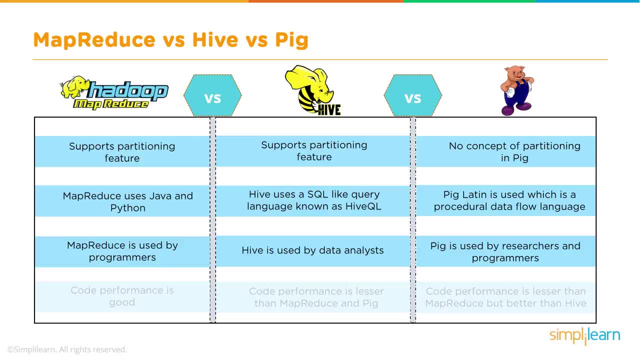 Programmers have been known to go in and use a Hive for a quick query And anybody's been able to use Pig for a quick query or research. Under Map and Reduce code performance is really good. Under Hive code performance is lesser than Map and Reduce in Pig. 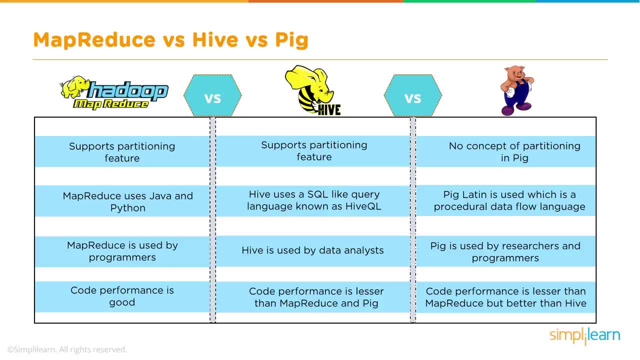 Under Pig code performance is lesser than MapReduce but better than Hive. So if we're going to look at speed and time, the MapReduce is going to be the fastest performance on all of those Where Pig will have second, and Hive follows in the back. 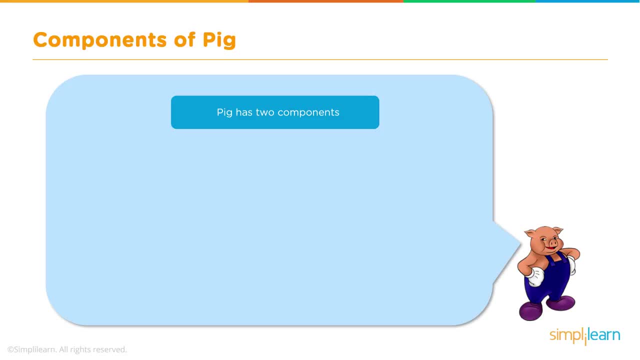 Let's look at components of Pig. Pig has two main components. We have Pig Latin. Pig Latin is a procedural data flow language used in Pig to analyze data. It is easy to program using Pig Latin. It is similar to SQL. And then we have the Runtime Engine. 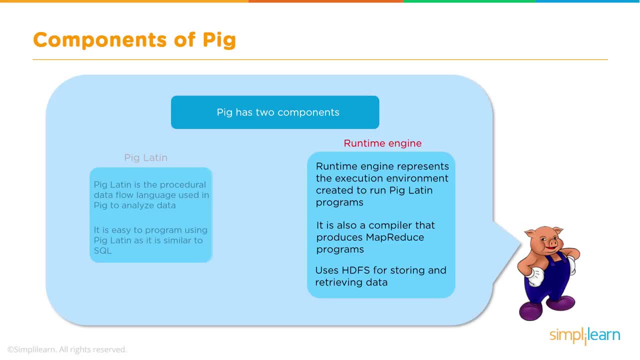 Runtime Engine represents the execution environment created to run Pig Latin programs. It is also a compiler that produces MapReduce programs. It uses HDFS or your Hadoop file system for storing and retrieving data, And as we dig deeper into the Pig architecture, we'll see that we have Pig Latin scripts. 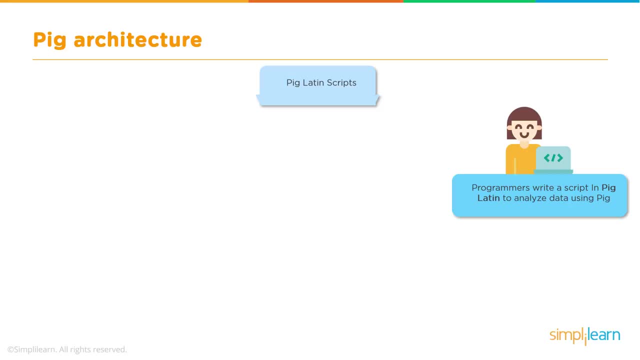 Programmers write a script in Pig Latin to analyze data using Pig. Then you have the Grunt shell And it actually says Grunt when we start it up- And we'll show you that here in a little bit- Which goes into the Pig server. 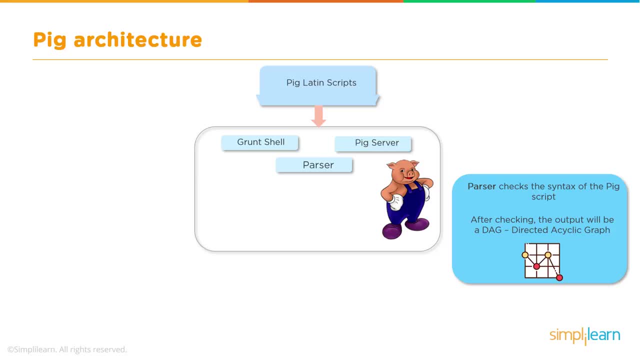 And this is where we have our parser. Parser checks the syntax of the Pig script. After checking, the output will be a DAG directed acylic graph. And then we have an optimizer Which optimizes. after your DAG, your logical plan is passed to the logical optimizer, where an optimization takes place. 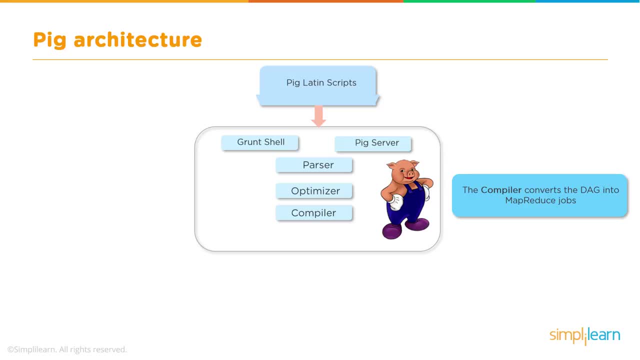 Finally, the compiler components. Finally, the compiler converts the DAG into MapReduce jobs And then that is executed on the MapReduce under the execution engine. The results are displayed using dump statement and stored in HDFS using store statement, And again, we'll show you that. 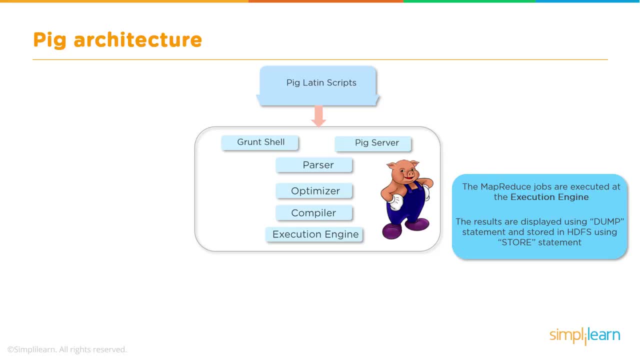 The kind of end you always want to execute everything once you've created it, And so dump is kind of our execution statement And you can see right here, as we were talking about earlier, once we get to the execution engine and it's coded into MapReduce. 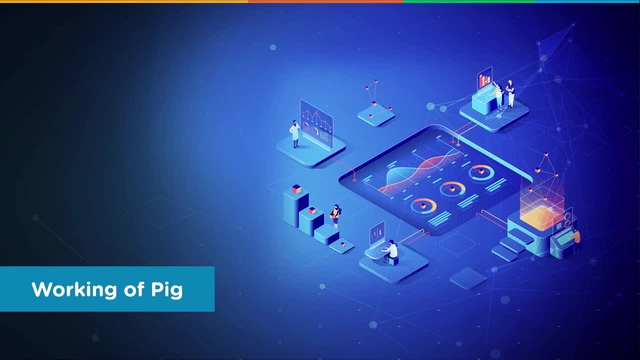 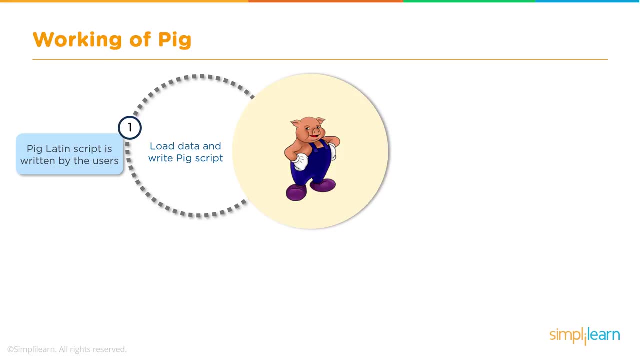 then the MapReduce processes it onto the HDFS. Working of Pig Pig Latin script is written by the users. So you have load data and write Pig script and Pig operations. So when we look at the working of Pig Pig Latin script is written by the users. 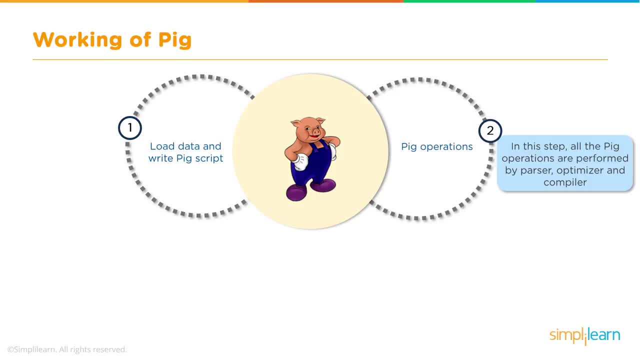 There's step one- We load data and write Pig script, And step two. in this step all the Pig operations are performed by parser, optimizer and compiler. So we go into the Pig operations And then we get to step three, execution of the plan. 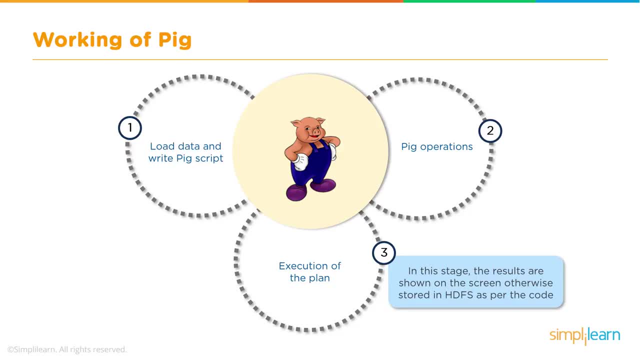 In this stage the results are shown on the screen, Otherwise stored in the HDFS as per the code. So it might be you have a small amount of data, you're reducing it to and you want to put that on the screen, Or you might be converting a huge amount of data which you want to put back into the Hadoop file system for other use. 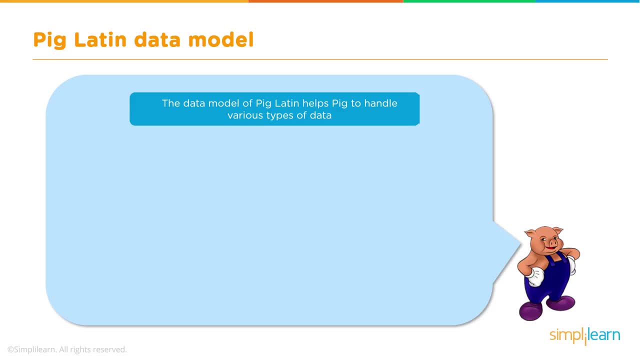 Let's take a look at the Pig Latin data model. The data model of Pig Latin helps Pig to handle various types of data. For example, we have Adam, Rob or 50. Adam represents any single value of primitive data type in Pig Latin, like integer, float string. 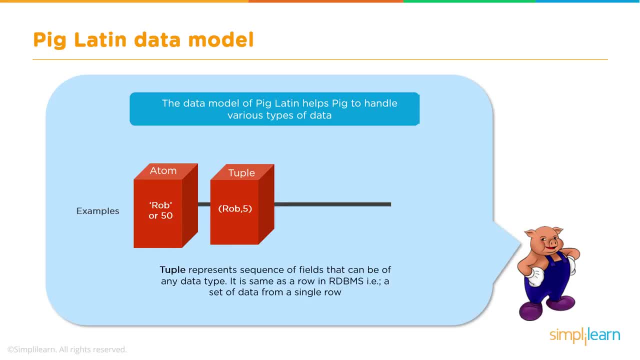 It is stored as a string. Then we have Tuple. So we go from our Adam, which is our most basic thing. So if you look at just Rob, or just 50, that's an Adam. That's our most basic object we have in Pig Latin. 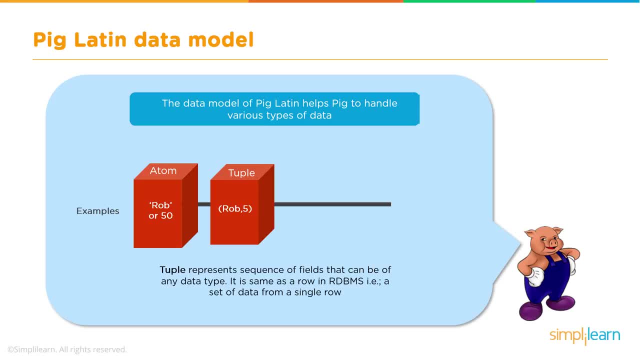 Then you have a Tuple. Tuple represents sequence of fields that can be of any data type. It is the same as a row in RDBMS, For example, a set of data from a single row And you can see, here we have Rob 5.. 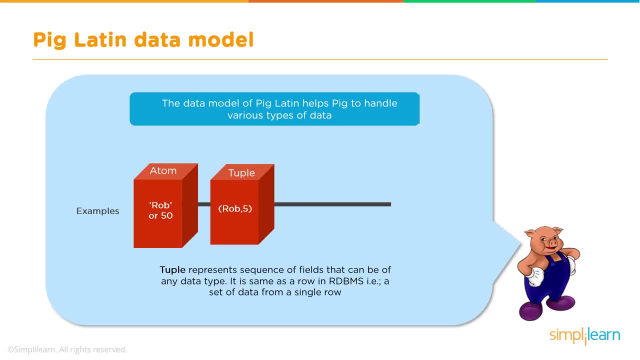 And you can imagine with many of our other examples we've used. you might have the ID number, the name where they live, their age, their date of starting the job. That would all be one row and stored as a Tuple, And then we create a bag. 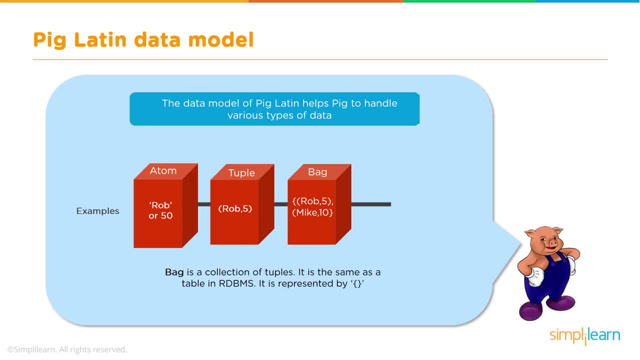 A bag is a collection of Tuples. It is the same as a table in RDBMS and is represented by brackets And you can see, here we have our table with Rob 5, Mike 10.. And we also have a map. 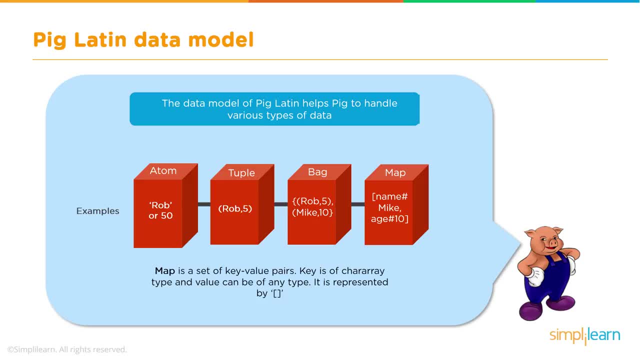 A map is a set of key-value pairs. Key is of character, array type, and a value can be of any type. It is represented by the brackets, And so we have name and age, Where the key value is Mike and 10.. Pig Latin has a fully nestable data model. 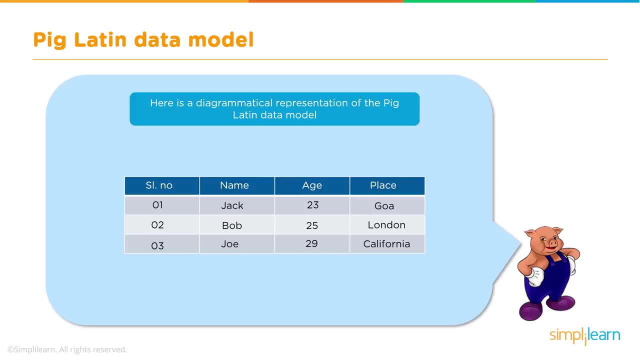 That means one data type can be nested within another. Here's a diagram representation of Pig Latin data model And in this particular example we have basically an ID number, a name, an age and a place, And when we break this apart, we look at this model from Pig Latin perspective. 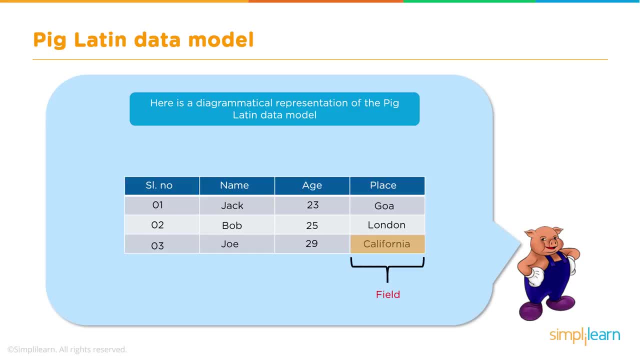 We start with our field And, if you remember, a field contains basically an atom. It is one particular data type And the atom is stored as a string, which then converts it into either an integer number or character string. Next we have our tuple. 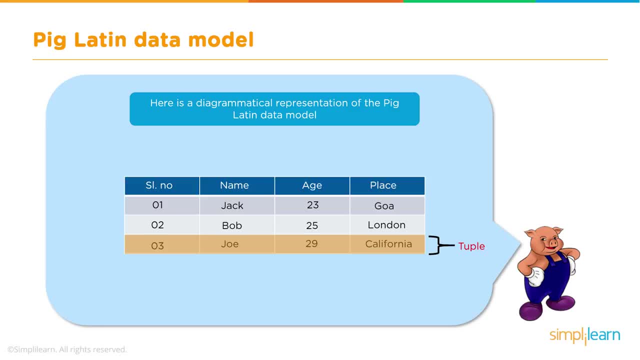 And in this case you can see that it represents a row. So our tuple would be 3, Joe, 29, California. And finally, we have our bag, which contains three rows in it in this particular example. Let's take a quick look at Pig execution modes. 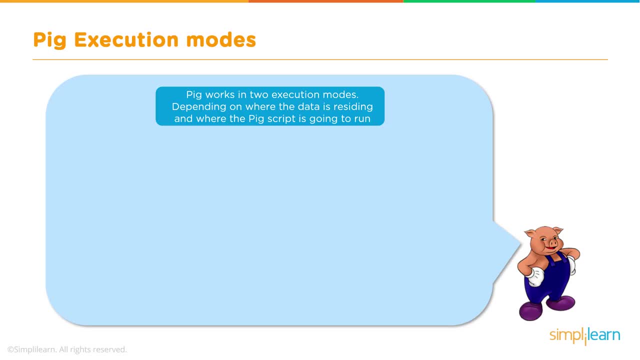 Pig works in two execution modes, depending on where the data is reciting and where the Pig script is going to run. We have local mode Here. the Pig engine takes input from the Linux file system and the output is stored in the same file system. 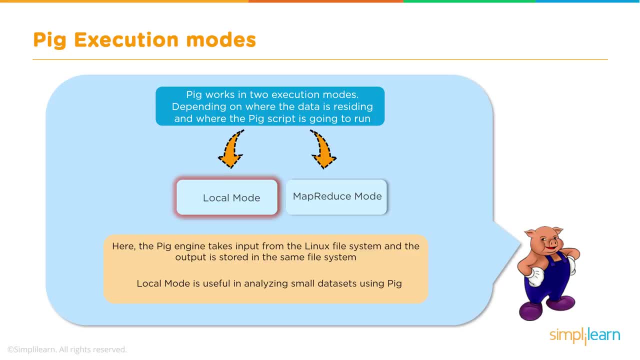 Local mode is useful in analyzing small data sets using Pig And we have the MapReduce mode. Here the Pig engine directly interacts and executes in HDFS and MapReduce. In the MapReduce mode, queries written in Pig Latin are translated into MapReduce jobs and are run on a Hadoop cluster. 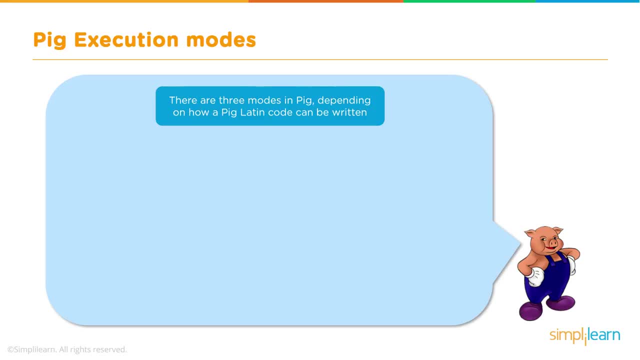 By default, Pig runs in this mode. There are three modes in Pig, Depending on how a Pig Latin code can be written. We have our interactive mode, batch mode and embedded mode. The interactive mode means coding and executing the script line by line. 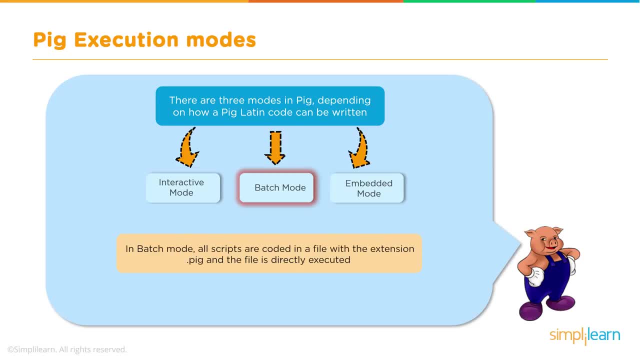 When we do our example, we'll be in the interactive mode. In batch mode, all scripts are coded in a file with the extension pig, and the file is directly executed. And then there's embedded mode. Pig lets its users define their own functions- UDFSs- in a programming language such as Java. 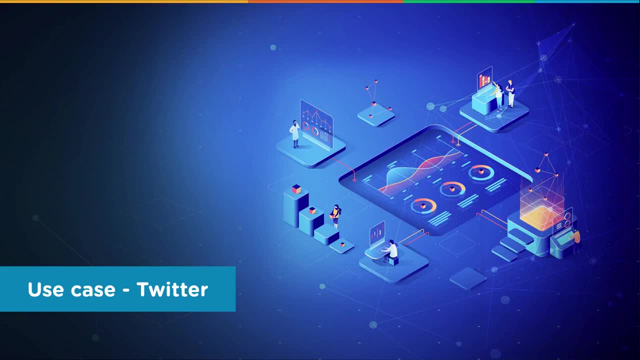 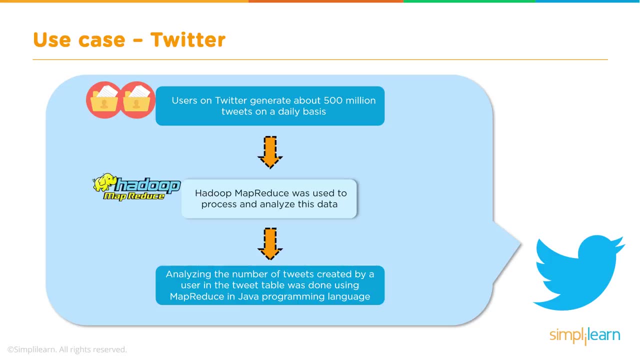 So let's take a look and see how this works in a use case. In this case, use case Twitter. Users on Twitter generate about 500 million tweets on a daily basis. The Hadoop MapReduce was used to process and analyze this data. 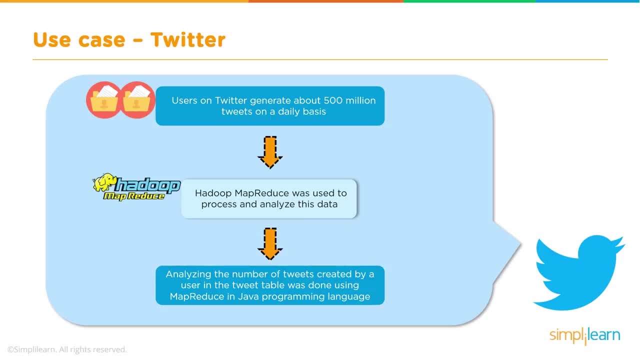 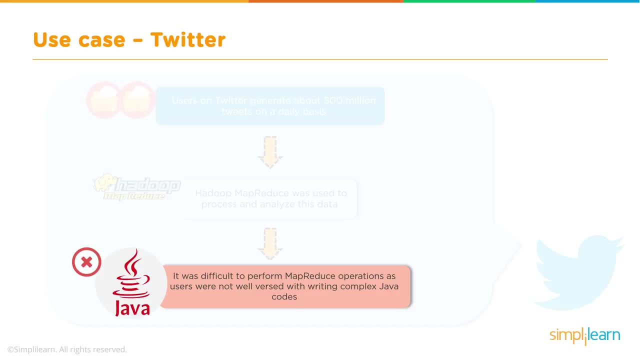 Analyzing the number of tweets created by a user in the tweet table was done using MapReduce in Java programming language, And you can see the problem. It was difficult to perform MapReduce operations as users were not well versed with written, complex Java codes. 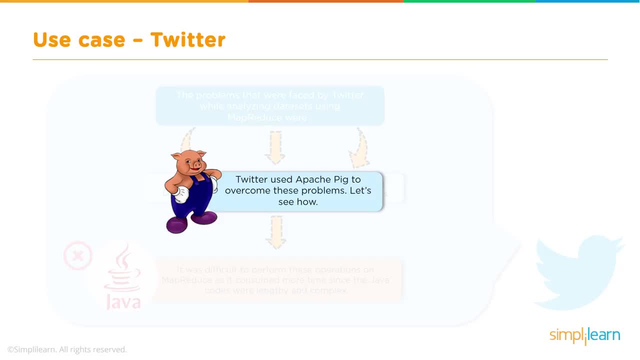 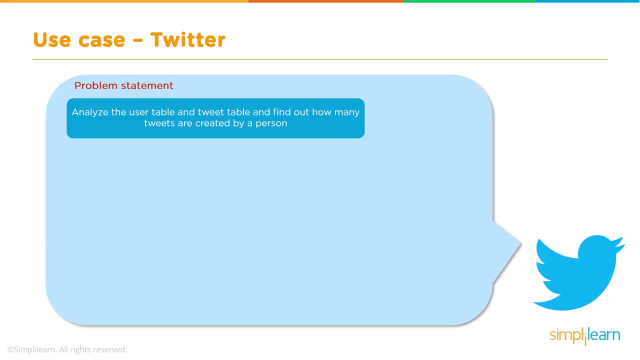 So Twitter used Apache Pig to overcome these problems. Let's see how. Let's start with the problem statement, Analyze the user table and tweet table and find out how many tweets are created by a person. And here you can see we have a user table. 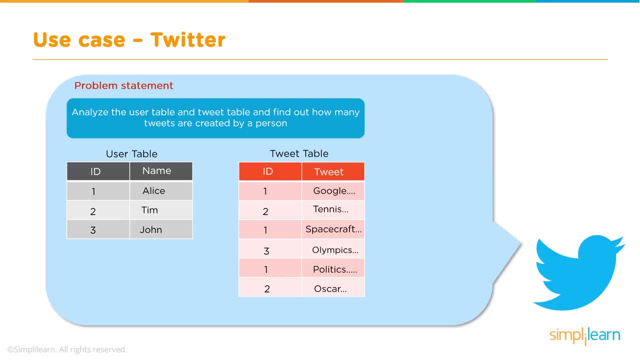 We have Alice, Tim and John with their ID numbers 1,, 2,, 3.. And we have a tweet table. In the tweet table you have the ID of the user and then what they tweeted. Google was a good whatever it was- tennis, dot dot dot, spacecraft, Olympics, politics- whatever they're tweeting about. 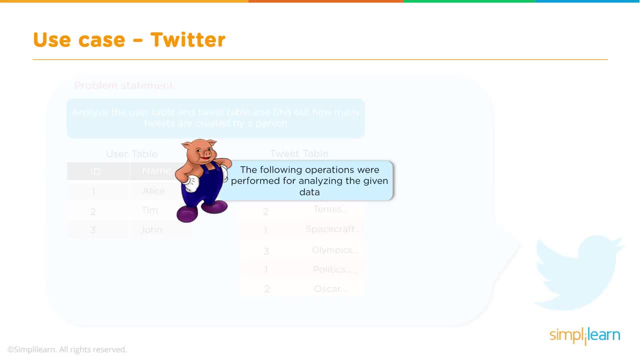 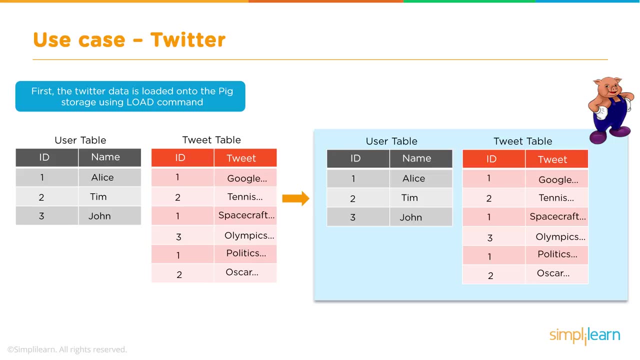 The following operations were performed for analyzing given data: First the Twitter data is loaded into the Pig server, Then the Twitter data is loaded into the Pig storage using load command And you can see here we have our data coming in and then that's going into Pig storage. 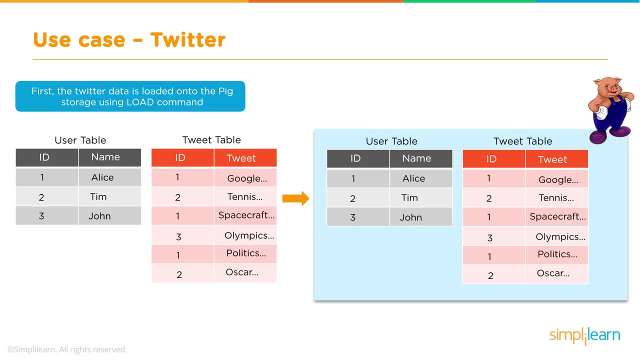 And this data is probably on an enterprise computer, So this is actually active Twitter's going on. and then it goes into Hadoop file system. Remember, the Hadoop file system is a data warehouse for storing data, And so the first step is we want to go ahead and load it into the Pig storage, into our data storage system. 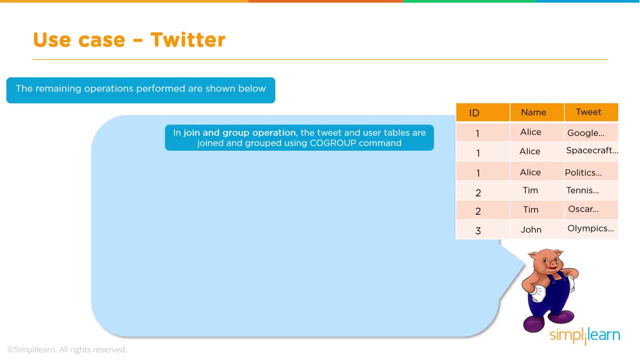 The remaining operations performed are shown below. In join and group operation the files are joined and grouped using co-group command And you can see here where we add a whole column when we go from user names and tweet to the ID linked directly to the name. 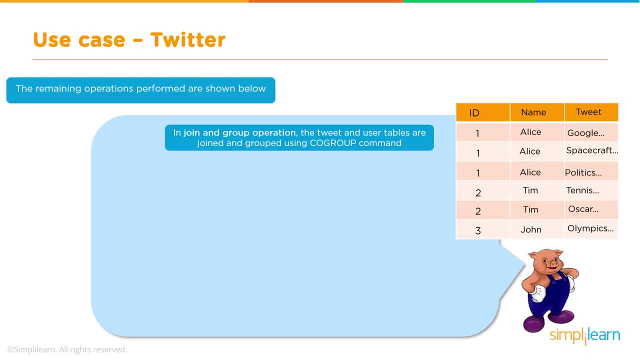 So Alice was user one, Tim was two and John three, And so now they're listed with their actual tweet. The next operation is the aggregation. The tweets are counted according to the names. The command used is count, So it's very straightforward. 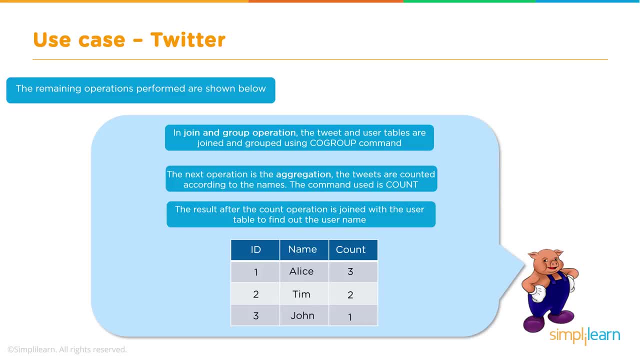 We just want to count how many tweets each user is doing And finally the result after the count operation is joined with the user table to find out the user name And you can see here where Alice had three, Tim two and John one. 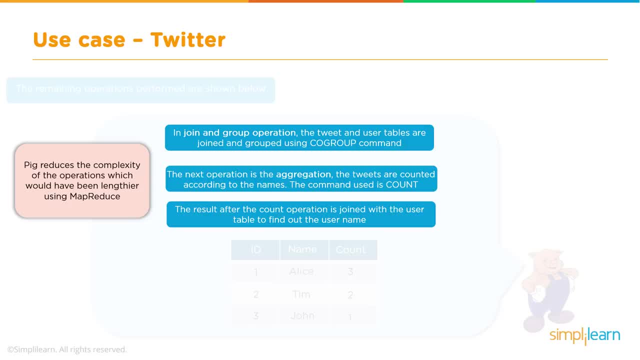 Pig reduces the complexity of the operations, which would have been lengthy, using MapReduce. In join and group operation, the tweet and user tables are joined and grouped using co-group command. The next operation is the aggregation. The tweets are counted according to the names. 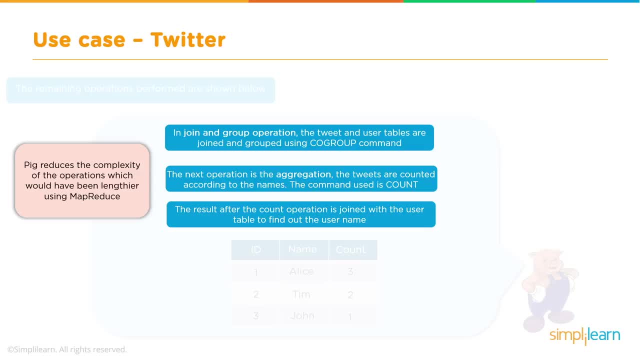 The command used is count. The result after the count operation is joined with the user table to find out the user name, And you can see we're talking about three lines of script versus a MapReduce code of about 80 lines. Finally, we could find out the number of tweets created by a user in a simple way. 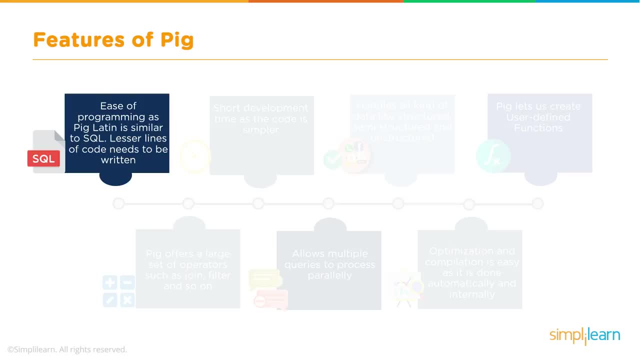 So let's go quickly over some of the features of Pig that we already went through. most of these First, ease of programming, as Pig Latin is similar to SQL. Lesser lines of code need to be written. Short development time, as the code is simpler. 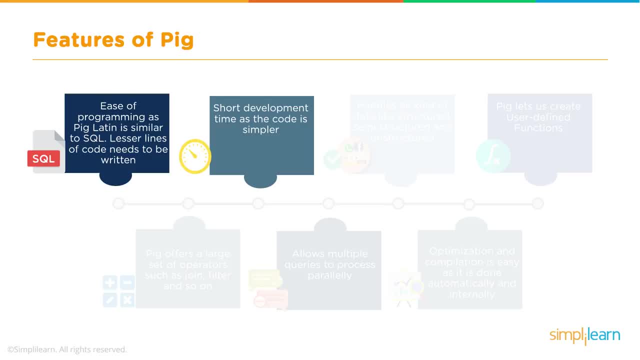 So we can get our queries out rather quickly instead of having to have a programmer spend hours on. it Handles all kind of data, like structured, semi-structured and unstructured. Pig lets us create user-defined functions. Pig offers a large set of operators such as join, filter and so on. 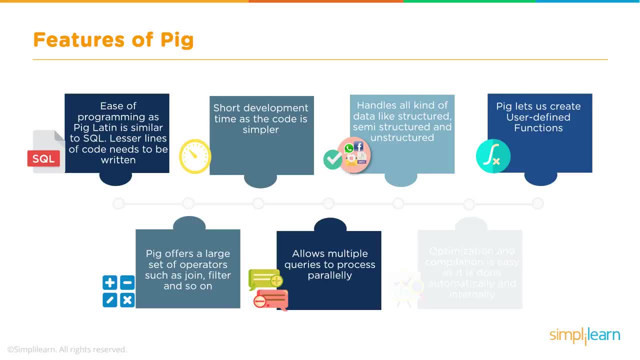 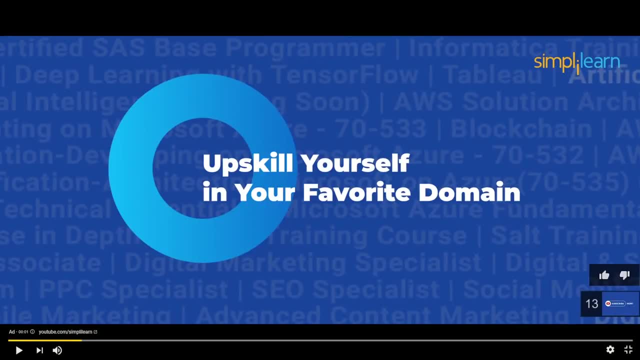 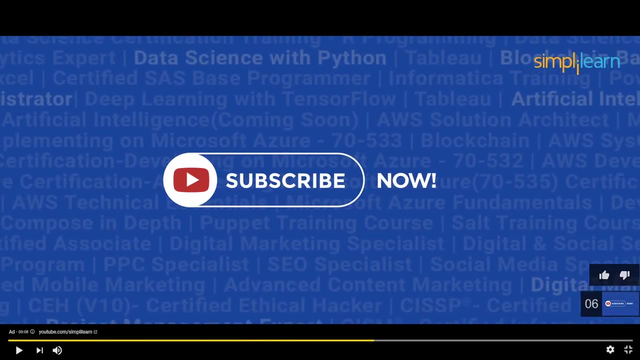 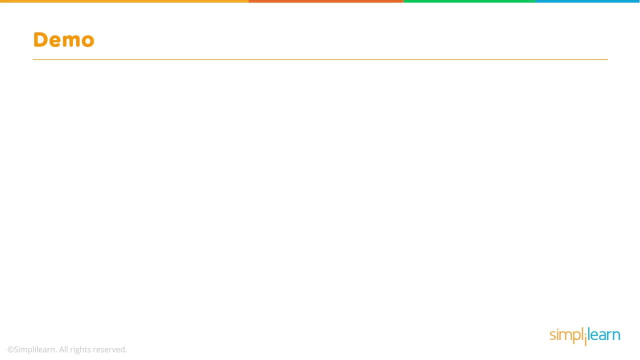 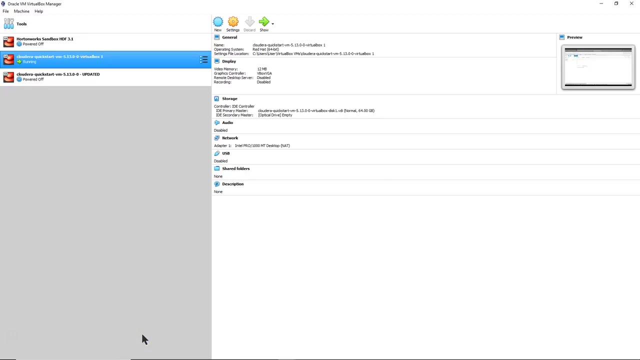 It allows for multiple queries to process unparallel, And optimization and compilation is easy, as it is done automatically and internally. So enough theory, Let's dive in and show you a quick demo on some of the commands you can do in Pig. Today's setup will continue as we have in the last three demos: to go ahead and use Cloudera Quickstart. 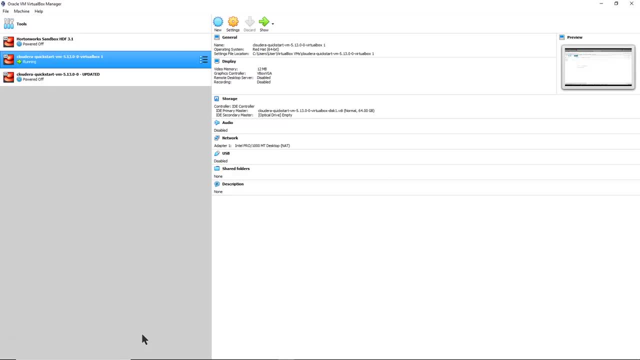 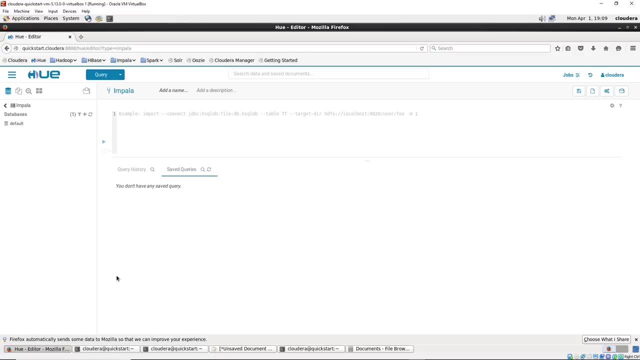 And we'll be doing this in VirtualBox. We do have a tutorial in setting that up. You can send a note to our Simply Learn team and they can get that link to you Once your Cloudera Quickstart has spun up. and remember this is VirtualBox. 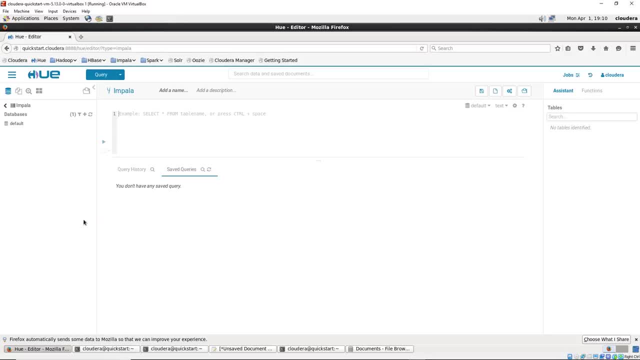 We've created a virtual machine, And this virtual machine is CentOS Linux. Once it's spun up, you'll be in a full Linux system here And, as you can see, we have Thunderbird Browser, which opens up to the Hadoop Basic System Browser. 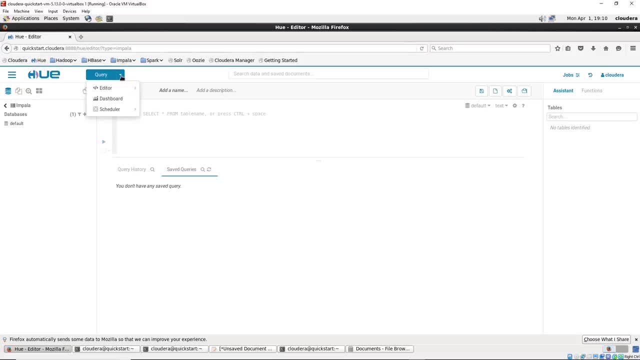 And we can go underneath the hue where it comes up by default. If you click on the pull-down menu and go under Editor, you can see there's our Impala, our Hive Pig, along with a bunch of other query languages you can use. 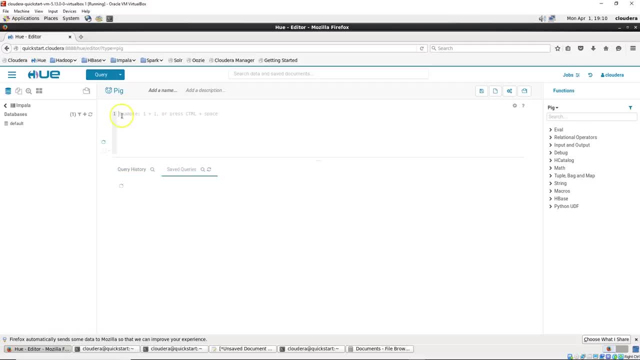 And we're going under Pig. And then, once you're in Pig, we can go ahead and use our command line here and just click that little blue button to start it up and running. We will actually be working in Terminal Window, And so if you were in the Cloudera Quickstart. 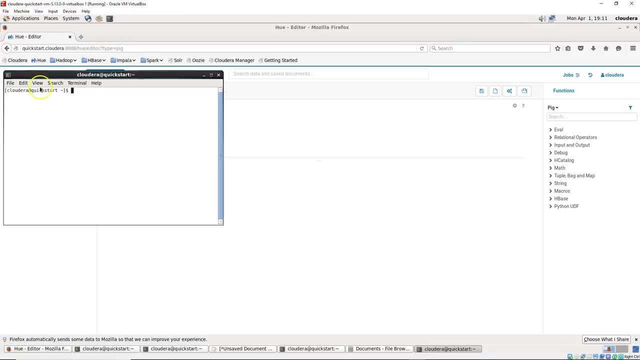 you can open up the Terminal Window up top, Or if you're in your own setup and you're logged in, you can easily use all of your commands here in Terminal Window And we'll zoom in. That way you get a nice view of what's going on. 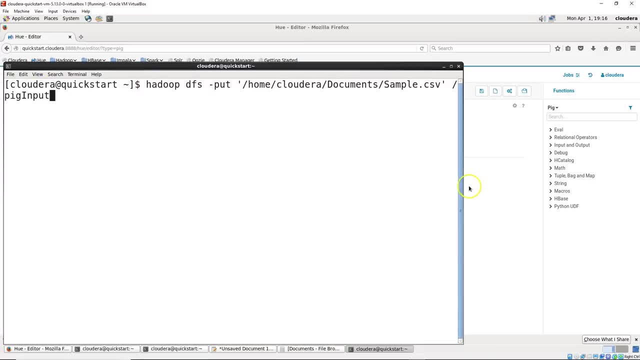 There we go Now for our first command. we're going to do a Hadoop command and import some data. We're going to import some data into the Hadoop system, in this case a Pig input. And let's just take a look at this. 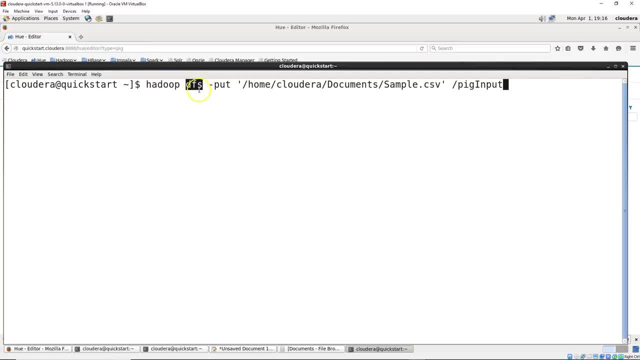 We have Hadoop Now let's just know it's going to be a Hadoop command- DFS. There's actually four variations of DFS, So if you have HDFS or whatever, that's fine. All four of them used to be different setups underneath different things. 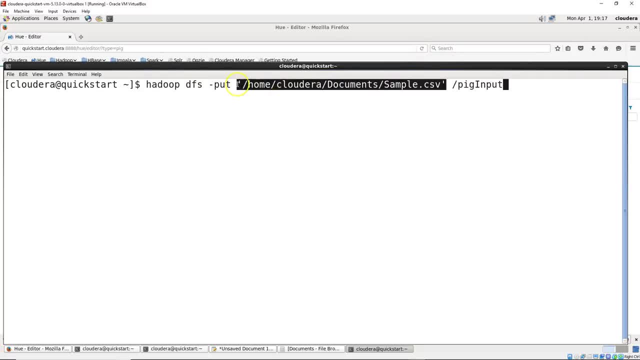 and now they all do the same thing And we want to put this file, which in this case is under Home, Cloudera, Documents and Sample, And we just want to take that and put it into the Pig input. And let's take a look at that file. 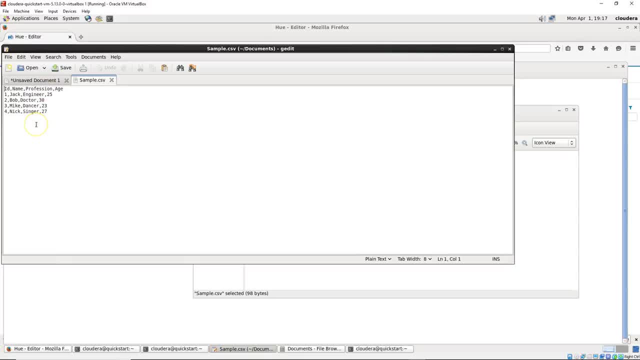 If I go into my document browsers and open this up, you'll see it's got a simple ID, name, profession and age. We have 1jackengineer25.. And that was in one of our earlier things we had in there. 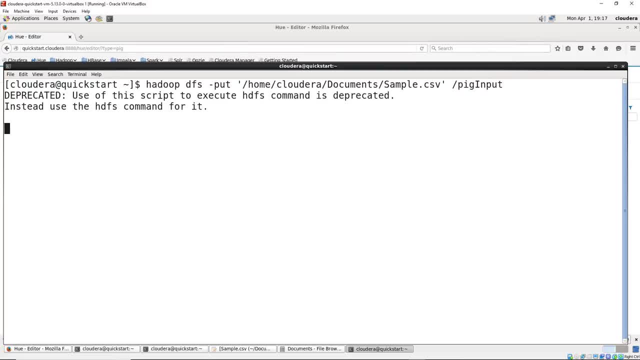 And so let's go ahead and hit Enter and execute this, And now we've uploaded that data and it's gone into our Pig input, And then a lot of the Hadoop commands mimic the Linux commands, And so you'll see we have cat as one of our commands. 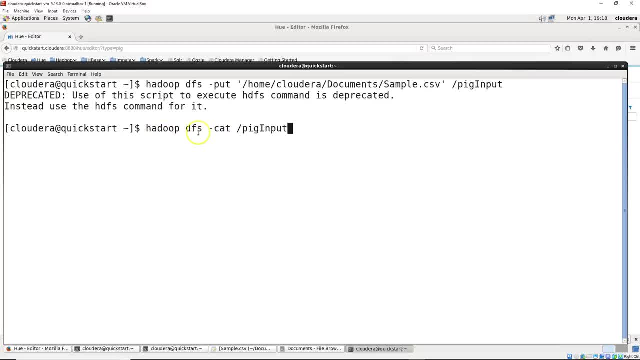 or it has a hyphen before it. So we execute that with Hadoop DFS hyphen- cat slash, pig input, because that's what we called it and that's where we put our sample CSV at And we execute this. You can see from our Hadoop system it's going to go in and pull that up. 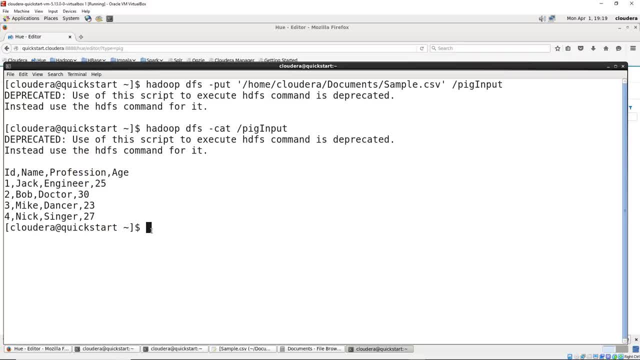 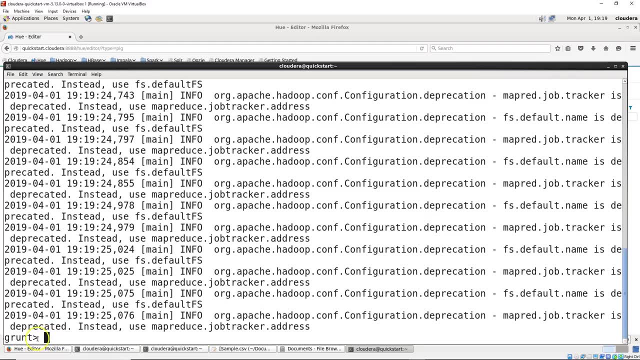 and, sure enough, it pulls out the data file we just put in there, And then we can simply enter the Pig Latin or Pig Editor mode by typing in pig And we can see here. by our grunt, I told you that's how it was going to tell you you were in Pig Latin. 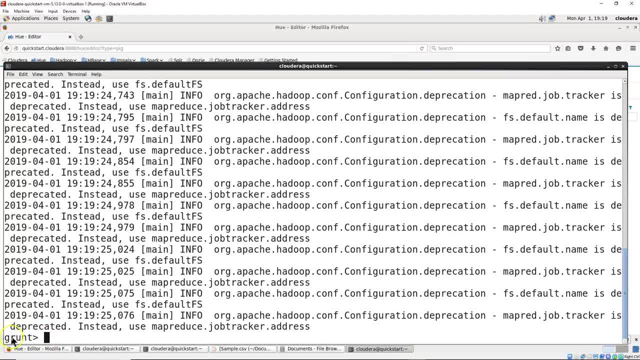 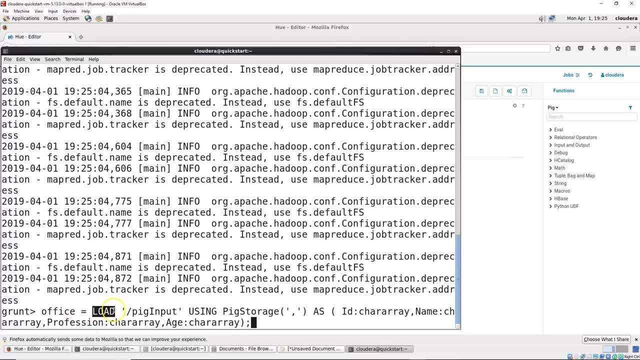 there's our grunt command line. So we are now in the Pig shell And then we'll go ahead and put our load command in here, And the way this works is I'm going to have office equals load. And here's my load. 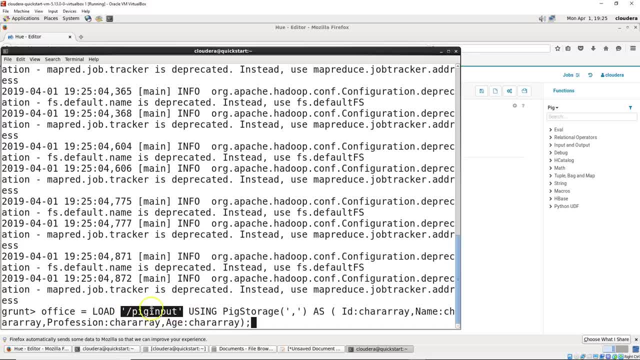 In this case it's going to be Pig input. We have that in single brackets, You remember. that's where the data is in the Hadoop file system, where we dumped it into there. We're going to be using Pig storage. Our data was separated as with a comma. 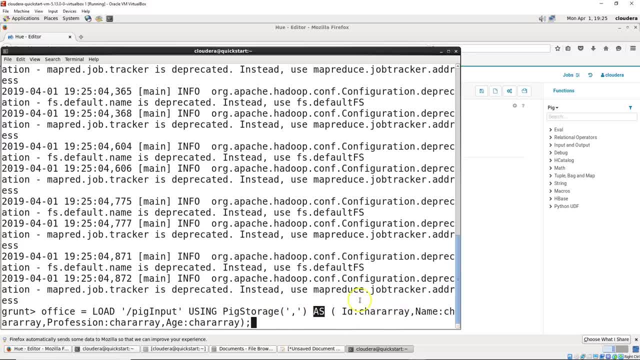 So there's our comma separator, And then we have as- And in this case we have an ID character array, name character array, profession character array and age character array, And we're just going to do them all as character arrays. 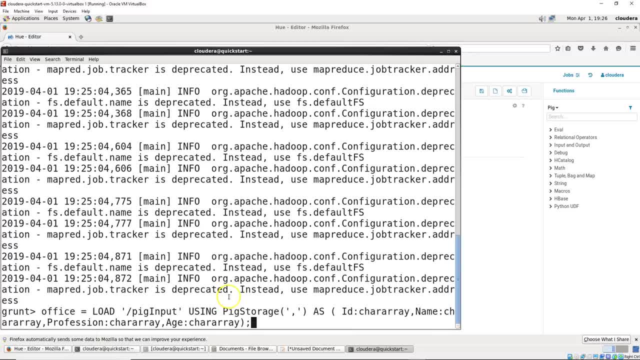 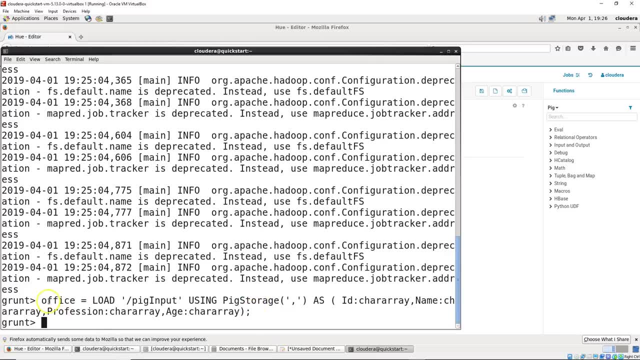 just to keep this simple for this one. And then when I hit put this all in here, you can see that's our full command line going in And we have our semicolon at the end. So when I hit enter, it's now set office up. 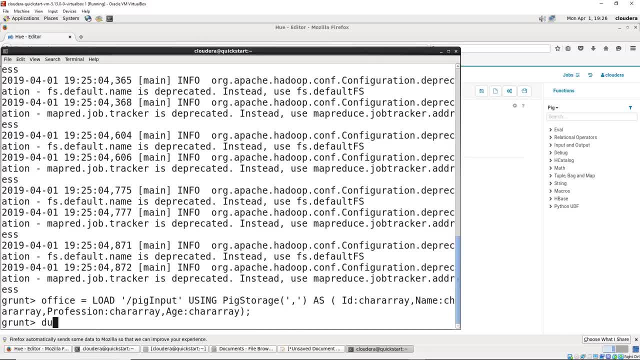 But it hasn't actually done anything yet. It doesn't do anything until we do dump office. So there's our command to execute whatever we've loaded or whatever setup we have in here. Now we run that. you can see it go through the different languages. 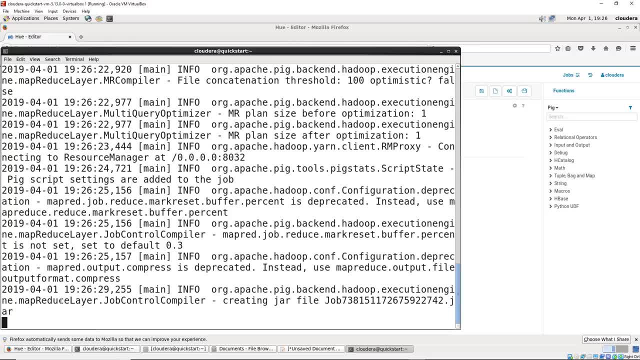 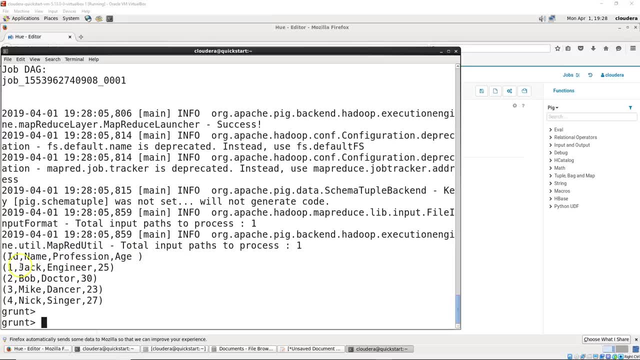 And this is going through the MapReduce. Remember we're not doing this locally, We're doing this on the Hadoop setup And once we've finished our dump, you can see we have ID, name, profession, age and all the information that we just dumped into our Pig. 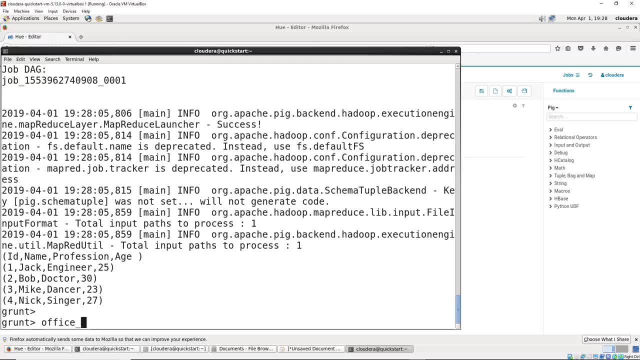 Now we can now do. let's say, oh, let's say we have a request, just for- we'll keep it simple in here, but just for the name and age, And so we can go office. we'll call it each as our variable. 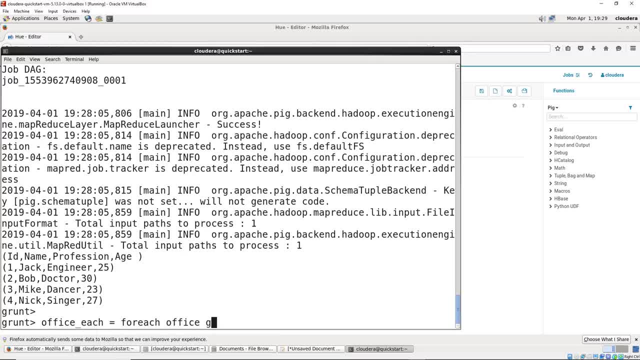 underscore each And we'll say: for each office: generate name, comma, age And for each means that we're going to do this for each row And if you're thinking MapReduce, you know that this is a map function Because it's mapping each row. 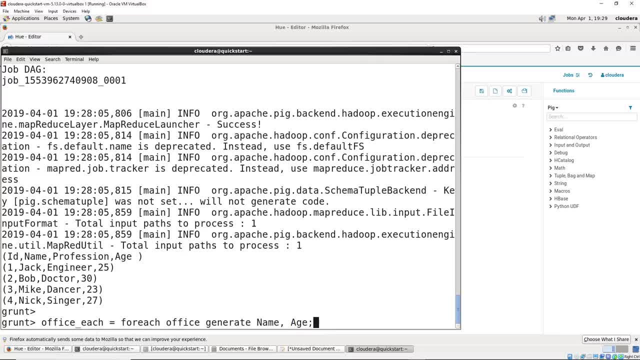 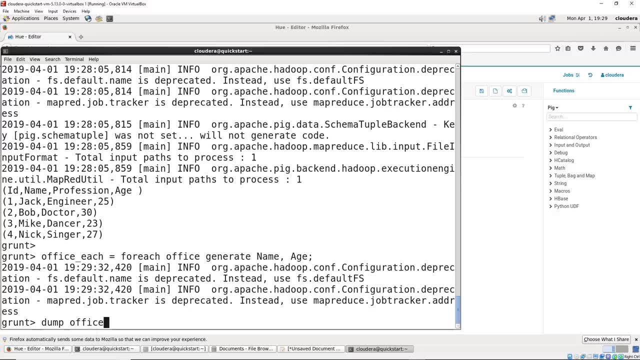 and generating name and age on here, And of course, we want to go ahead and close it with a semicolon. And then, once we've created our query or the command line in here, let's go ahead and dump office underscore, each in with our semicolon. 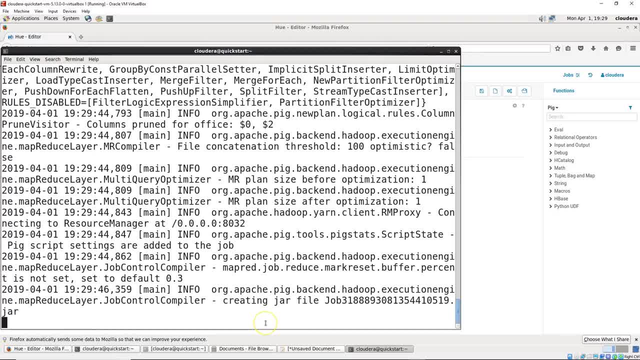 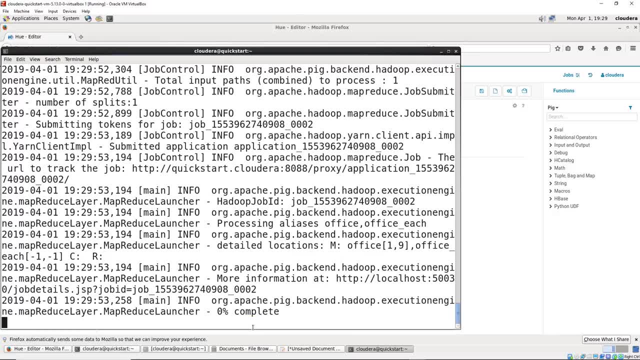 And this will go through our MapReduce setup on here, And if we were on a large cluster, the same processing time would happen. In fact, it's really slow because I have multiple things on this computer and this particular virtual box is only using a quarter of my processor. 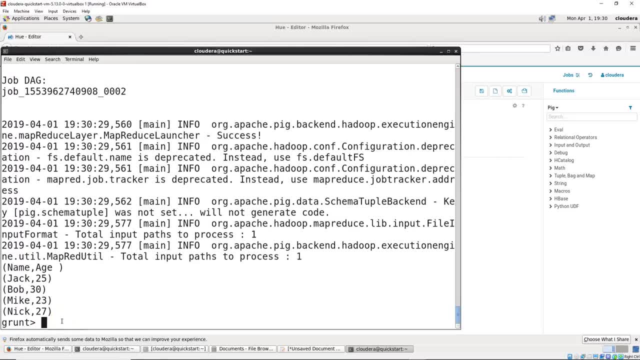 It's only dedicated to this And you can see here. there it is name and age, And it also included the top row, since we didn't delete that out of there or tell it not to, And that's fine for this example. 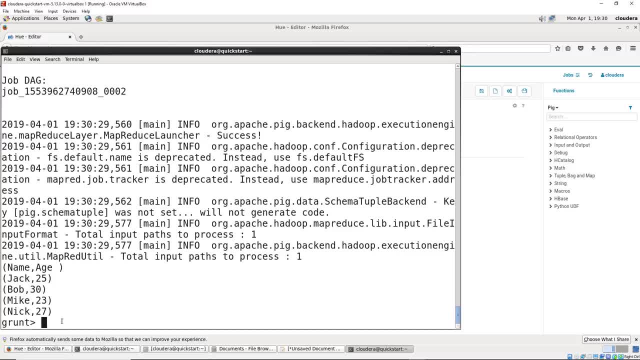 But you need to be aware of those things. when you're processing a significantly large amount of data, or any data, Then we can also do office and we'll call this DSC for descending. So maybe the boss comes to you and says, hey, can we order office by ID descending. 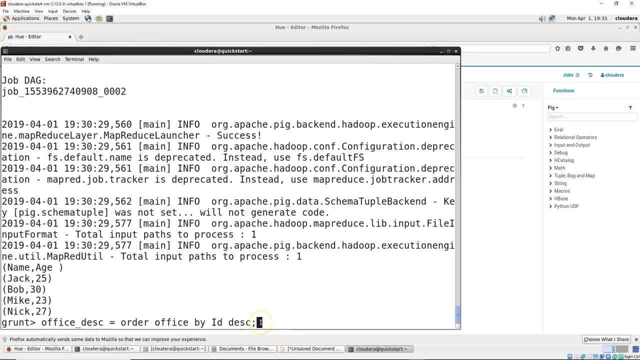 And, of course, your boss, you've taught them how. to your shareholder. it sounds a little derogatory when I say: boss, You've talked to the shareholder and you said: and you've taught them a little bit of pig Latin, and they know that they can now create office description. 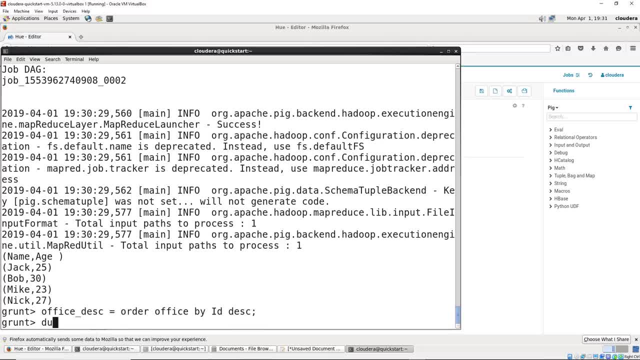 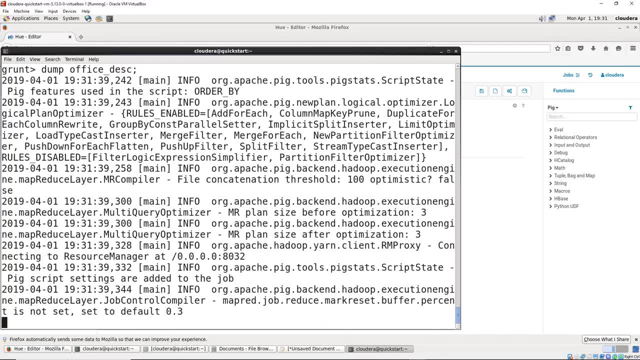 And we can order office by ID description And of course, once we do that we have to dump office underscore description so that it'll actually execute. And there it goes into our map reduce. It'll take just a moment for it to come up. 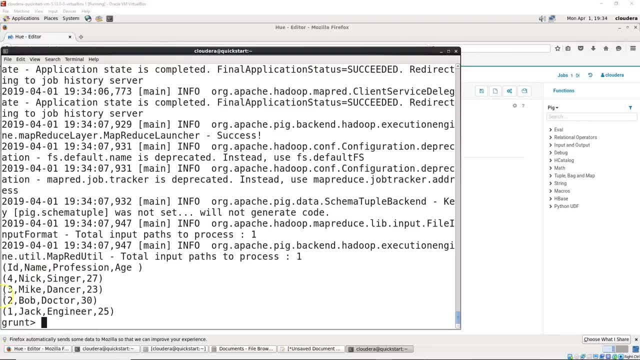 because, again, I'm running on only a quarter of my processor And you can see we now have our IDs in descending order returned. Let's also look at- and this is so important with any time you're dealing with big data- Let's create office with a limit. 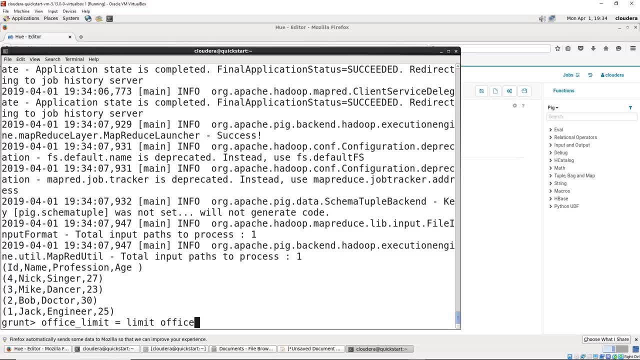 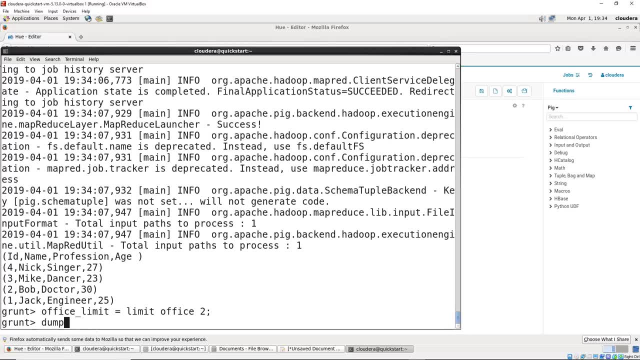 And you can of course, do any of this instead of with office. we could do this with office descending, So you get just the top two IDs on there. We're going to limit just to two And of course, to execute that we have to dump office underscore limit. 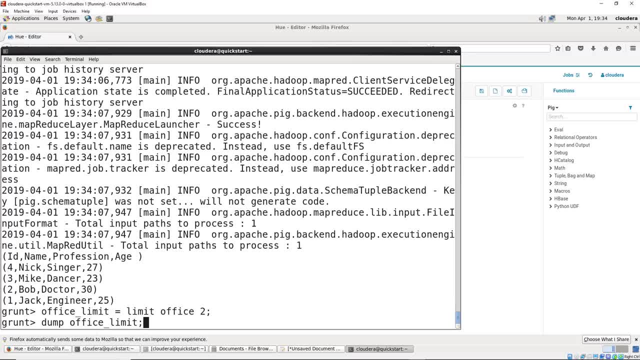 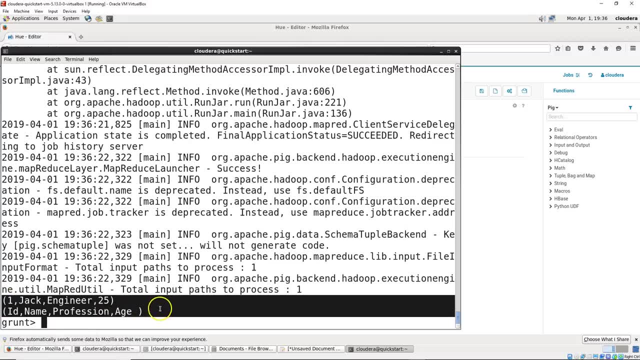 And you can just think of dumping your garbage into the pig pen for the pig to eat. There we go, Dump office limit two And that's going to just limit our office to the top two And for our output we get our first row. 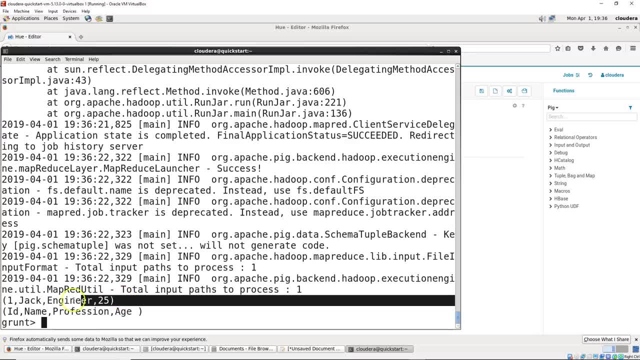 which had our ID, name, profession and age, And our second row, which is Jack, who's an engineer. And let's do a filter. We'll call it office underscore filter, You guessed it. Equals filter office by. 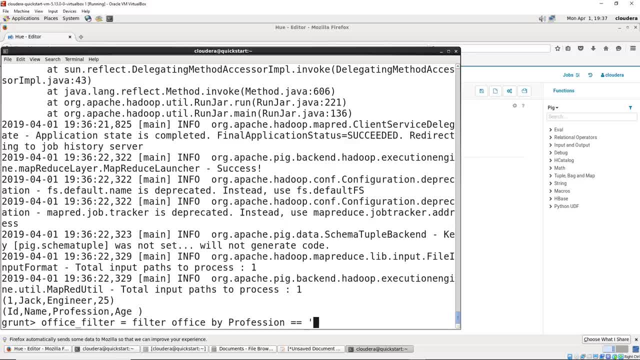 profession equals. And keep note this is similar to how Python does it with the double equal signs for equal, for doing a true false statement. So for your logic statement, remember to use two equal signs in pig And we're going to say it equals doctor. 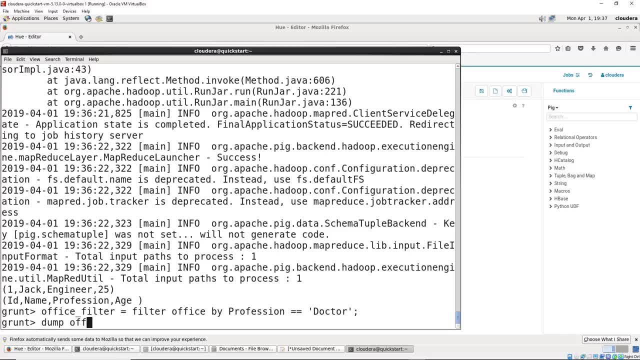 So we want to find out how many doctors do we have on our list? And we'll go ahead and do our dump. We're dumping all our garbage into the pig pen And we're letting pig take over and see what it can find out. 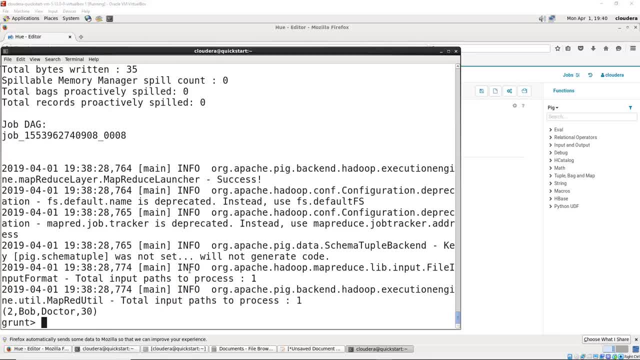 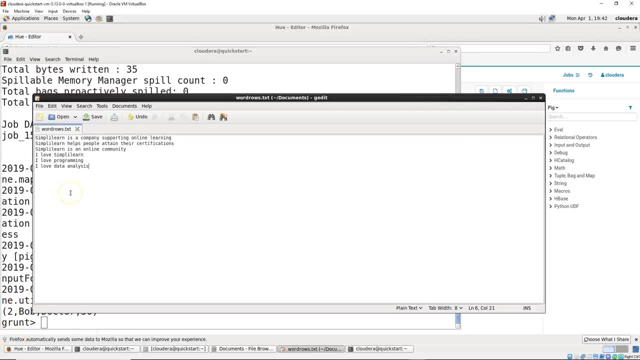 and see who's a doctor on our list And we find employee ID number two. Bob is a doctor, 30 years old. For this next section, we're going to cover something we see a lot nowadays in data analysis, And that's word counting. 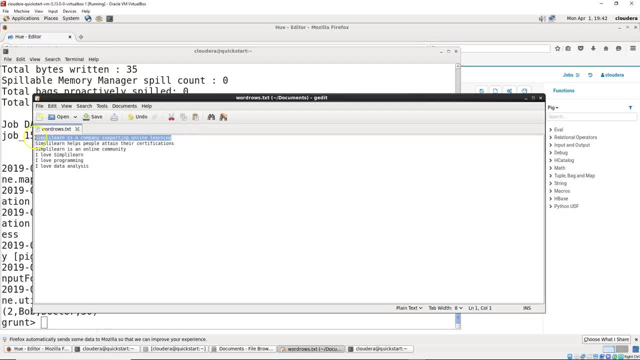 tokenization. That is one of the next big steps as we move forward in our data analysis, where we go from say, stock market analysis of highs and lows and all the numbers, to what are people saying about companies on Twitter? What are they saying on the web pages? 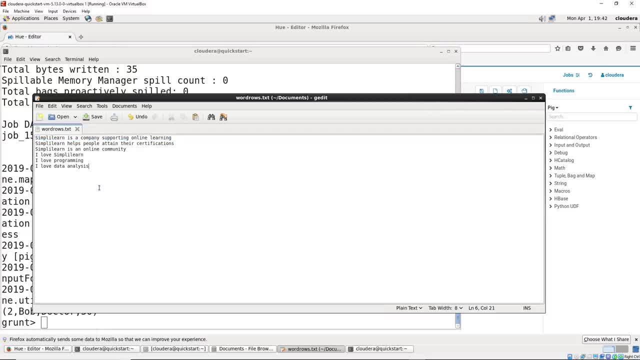 and on Facebook. Suddenly, you need to start counting words and finding out how many words are totaled, how many are in the first part of the document, and so on. We're going to cover a very basic word count example And in this case, 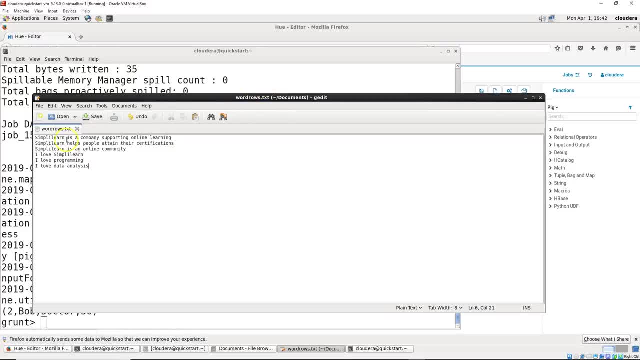 I've created a document called wordrowstxt And you can see here we have. SimplyLearn is a company supporting online learning. SimplyLearn helps people attain their certifications. SimplyLearn is an online community. I love SimplyLearn. I love programming. I love data analysis. 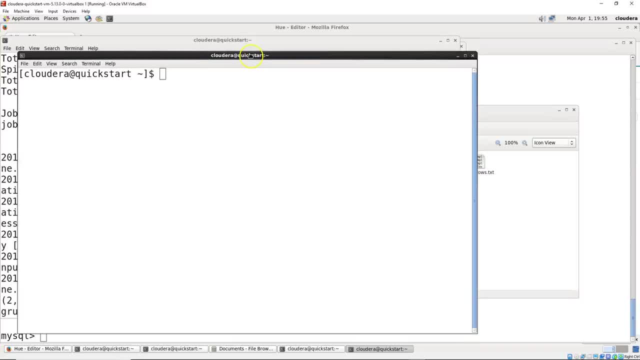 And I went and saved this into my documents folder so we could use it. And let me go ahead and open up a new terminal window for our word count. Let me go ahead and close the old one, So we're going to go in here. 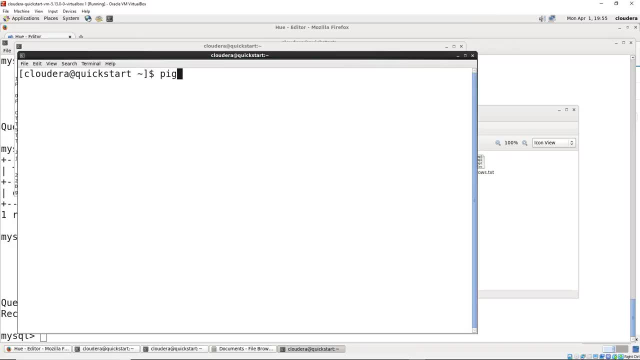 and instead of doing this as pig, we're going to do pig minus x local, And what I'm doing is I'm telling the pig to start the pig shell, but we're going to be looking at files local to our virtual box or this CentOS machine. 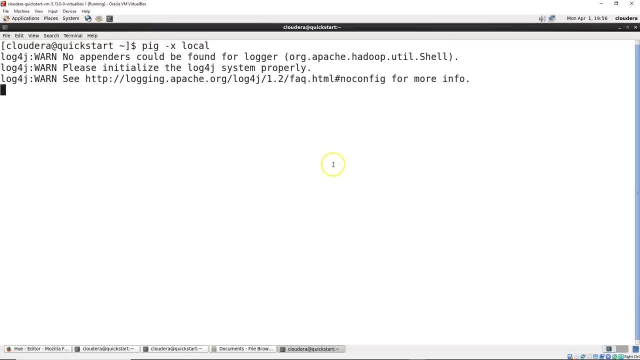 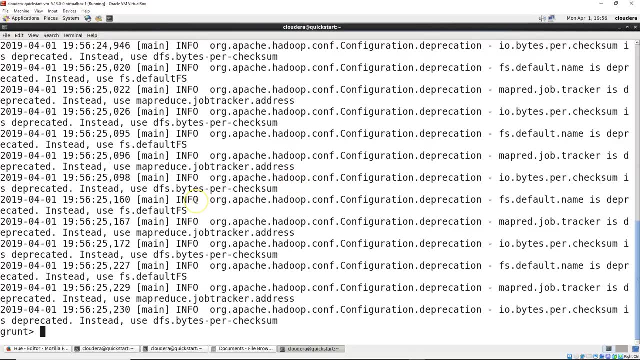 And let me go ahead and hit enter on there. Just maximize this up. There we go And it'll load pig up and it's going to look just the same as the pig. This is the pig we were doing, which was defaulted to our Hadoop system. 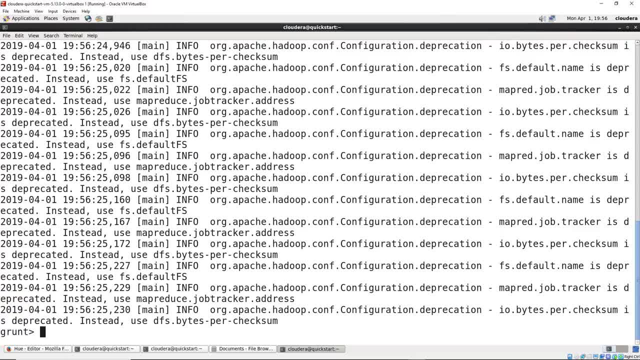 to our HDFS. This is now defaulted to the local system And now we're going to create lines, We're going to load it straight from the file. Remember last time we took the HDFS and loaded it into there and then loaded it into pig. 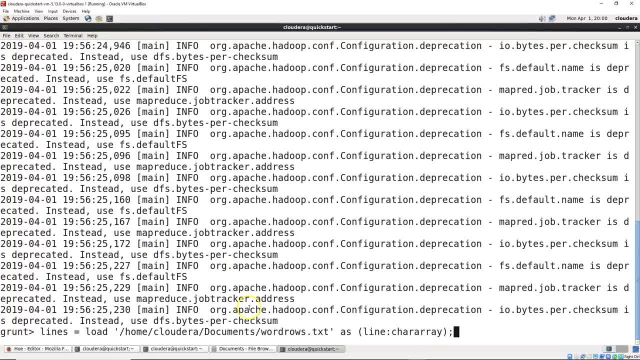 Since we've gone the local, we're just going to run a local script. We have lines equals: load home the actual full path home Cloudera documents, And I called it: word rows, dot text And as line is a character array. 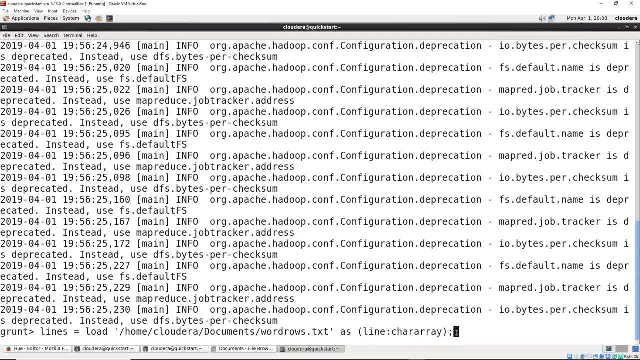 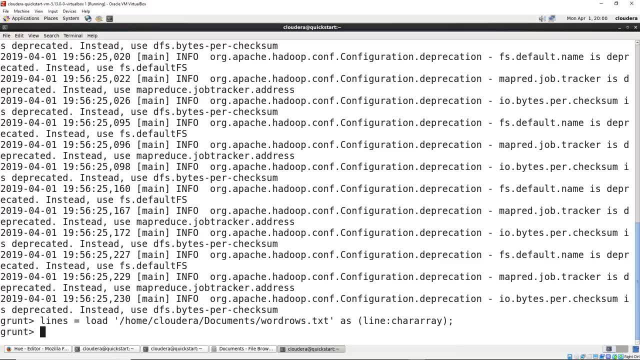 so each line, and I've actually- you can change this- to read each document. I certainly have done a lot of document analysis And then you go through and do word counts and different kind of counts in there. So once we go ahead and create our line, 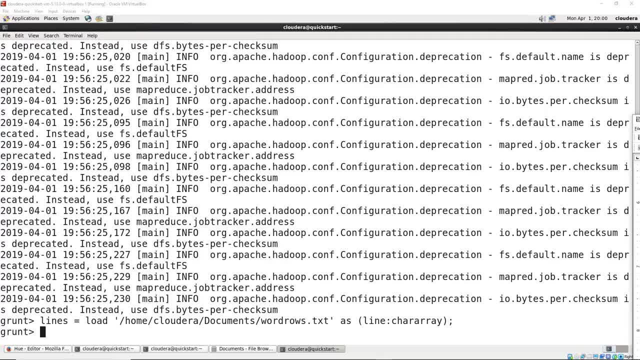 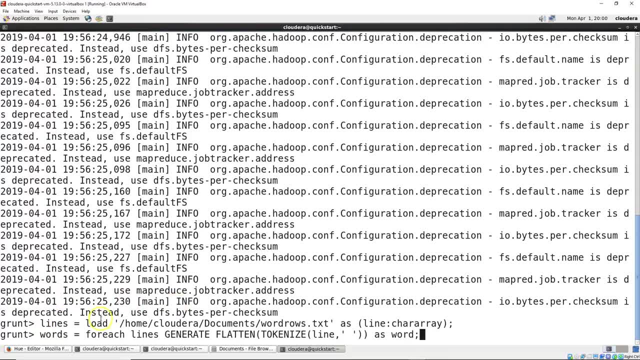 instead of doing the dump, we're going to go ahead and start entering all of our different setups or each of our steps we want to go through. And let's just take a look at this next one, because the load is straightforward: We're loading from this particular file. 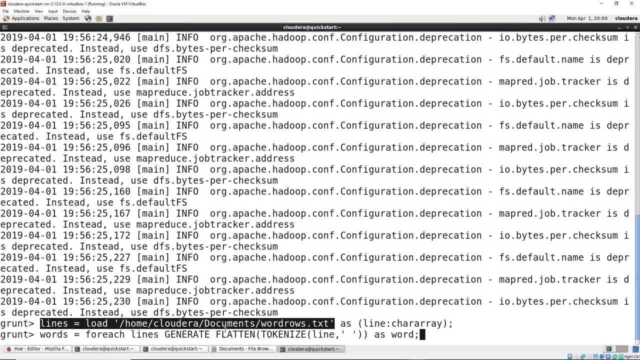 Since we're local, it's loading it directly from here instead of going into the Hadoop file system, And it says as: and then each line is read as a character array. Now we're going to do words equal for each of the lines. 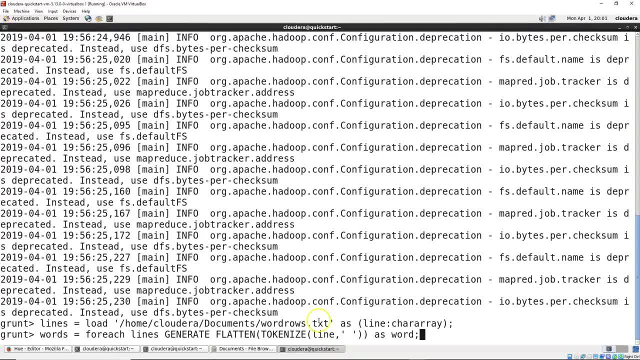 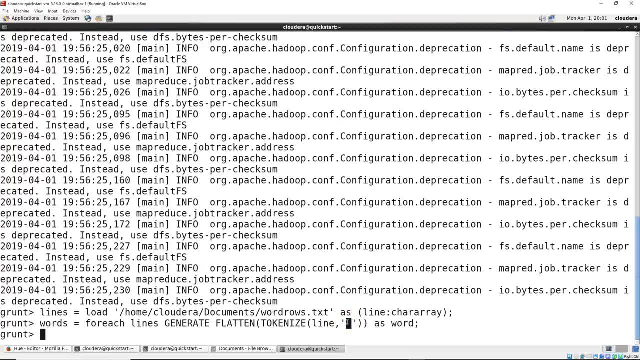 generate flat. tokenize line space as word. Now, there's a lot of ways to do this. This is if you're a programmer, you're just splitting the line up by spaces. There's actual ways to tokenize it. You got to look for periods. 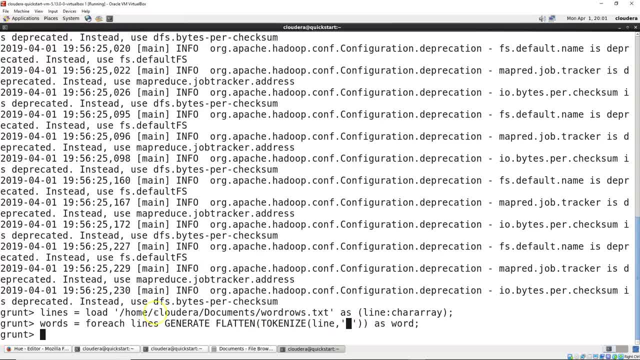 capitalization. There's all kinds of other things you play with with this, But for the most basic word count we're just going to separate it by spaces. The flatten takes some and just creates a. it flattens each of the words out. 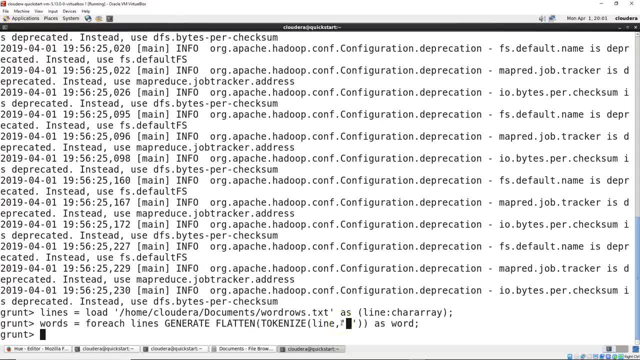 So this is: we're just going to generate a bunch of words for each line, And then each of those words is, as a word, A little confusing in there, but if you really think about it, we're just going down each line. 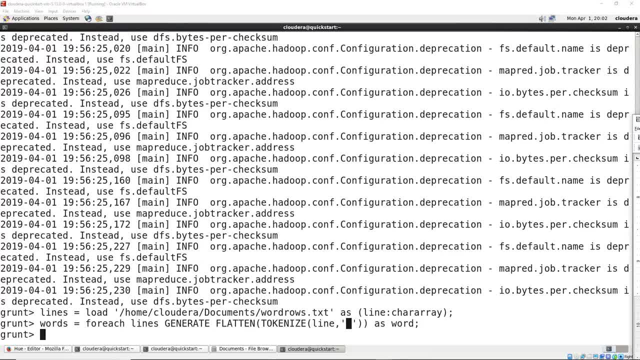 separating it out and we're generating a list of words. One thing to note is the default for tokenize. You can just do tokenize line without the space in there. If you do that, it'll automatically tokenize it by space. You can do either one. 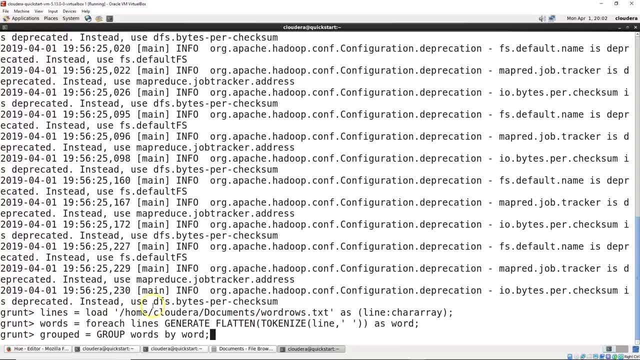 And then we're going to do group, We're going to group it by words. So we're going to group words by word. So when we split it up, each token is a word and it's a list of words, And so we're going to. 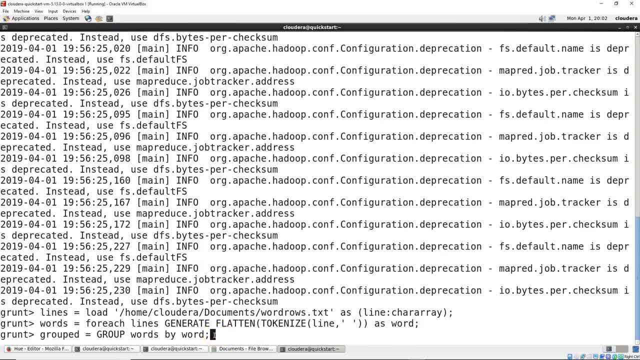 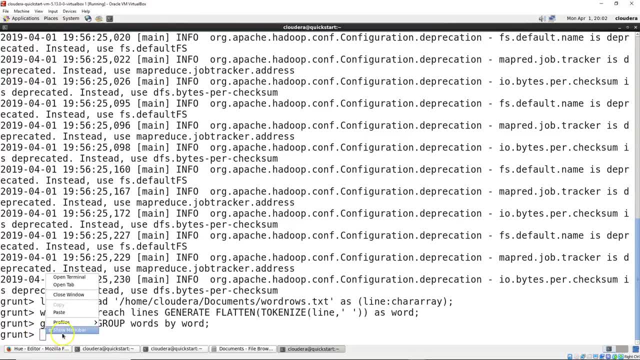 grouped equals group words by words. So we're going to group all the same words together, And if we're going to group them, then we want to go ahead and count them. And so for count, we'll go ahead and create a word count variable. 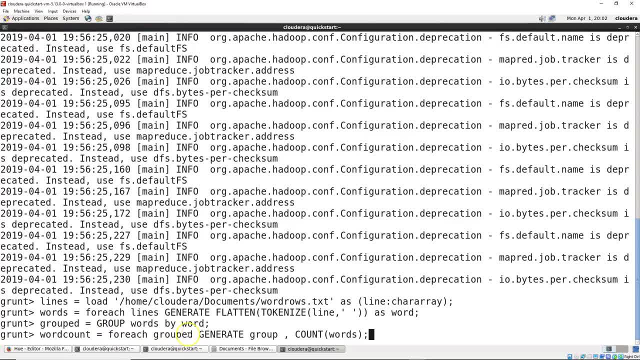 And here's our for each. So for each grouped. grouped is our line where we group all the words in the line that are similar. We're going to generate a group And then we're going to count the words For each grouped. 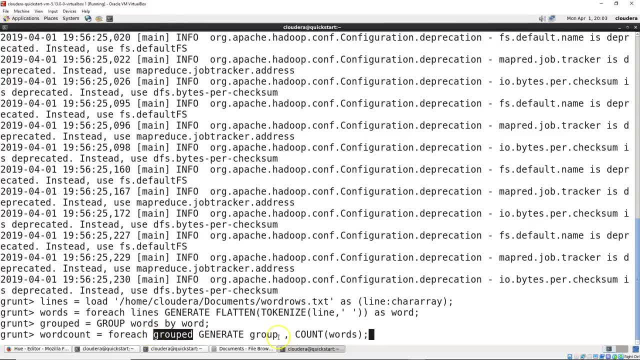 so for each line where we group the words together, we're going to generate a group and that's going to count the words. We want to know the word count in each of those And that comes back in our word count. And finally, 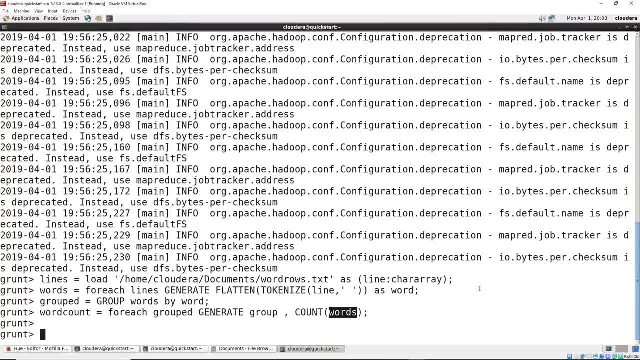 we want to take this and we want to go ahead and dump word count, And this is a little bit more what you see when you start looking at grunt scripts. You'll see right here these lines, right here we have each of the steps. 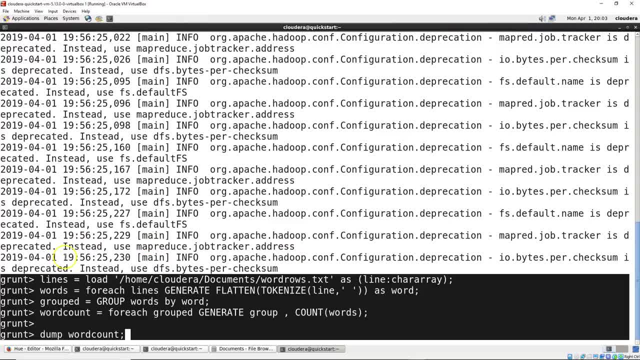 you take to get there. So we load our file For each of our lines, we're going to generate and tokenize it into words. Then we're going to take the words and we're going to group them by same words For each grouped. 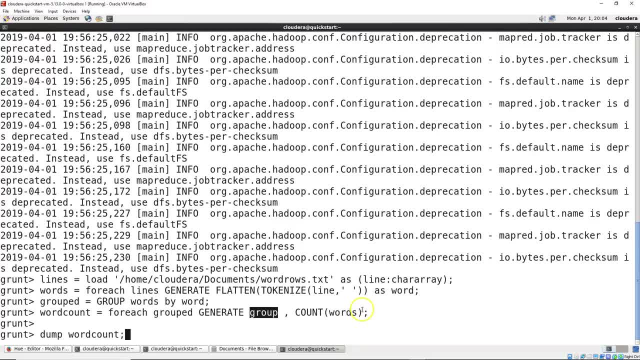 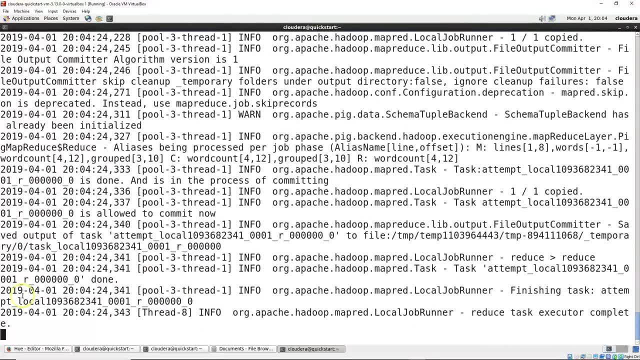 we're going to generate a group and we're just going to count the words. So we're going to summarize all the words in here And let's go ahead and do our dump word count, which executes all this And it goes through our MapReduce. 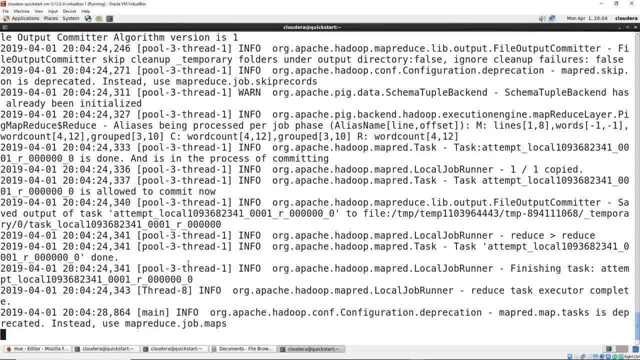 It's actually a local runner. You'll see down here. you start seeing where they still have MapReduce. but it's a special runner. We're mapping it. That's a part of each row being counted and grouped, And then when we do, 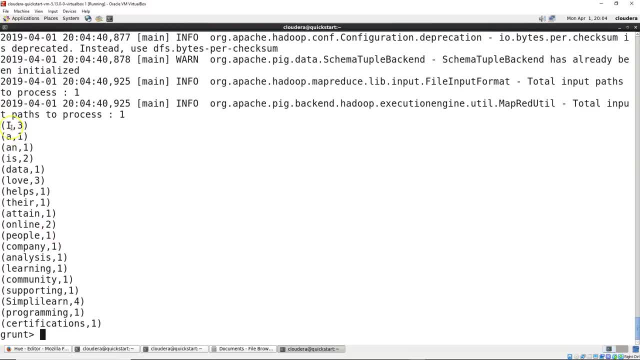 the word count, that's the reducer. The reducer creates these keys And you can see I is used three times: A came up once, N came up. once Is two. Continue on down here to attain online people company. 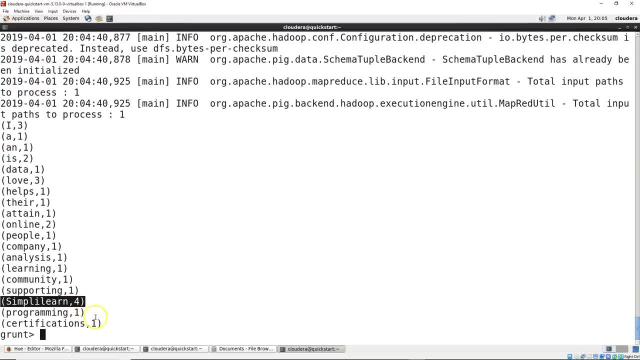 analysis simply learn. They took the top rating with four Certification. So all these things are then counted in how many words are used And in data analysis. this is probably the very, the very beginnings of data analysis where you might look at it. 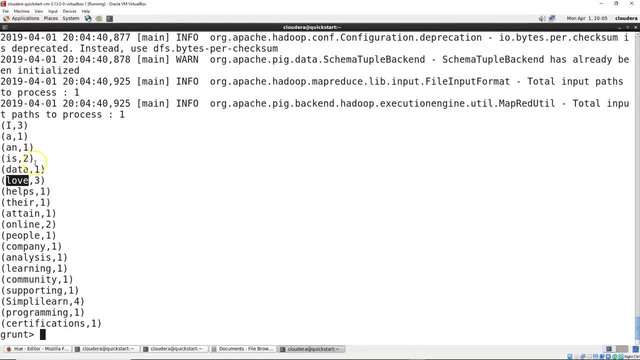 and say, oh, they mentioned love three times. So whatever's going on in this post, it's about love And what do they love? And then you might attach that to the different objects in here, So you can see that Pig Latin. 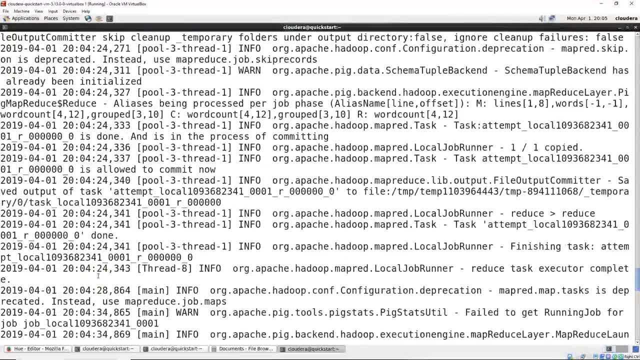 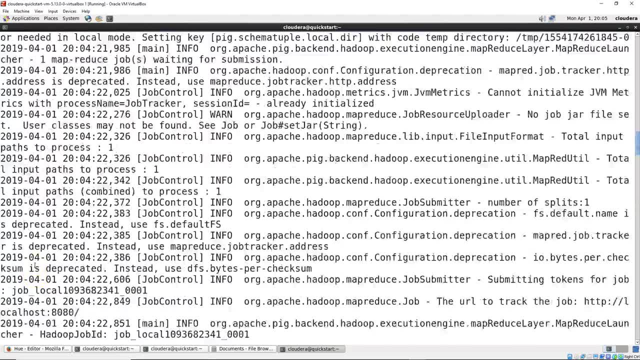 is fairly easy to use. There's nothing really. you know, it takes a little bit to learn the script, depending on how good your memory is. As I get older, my memory leaks a little bit more, so I don't memorize it as much. 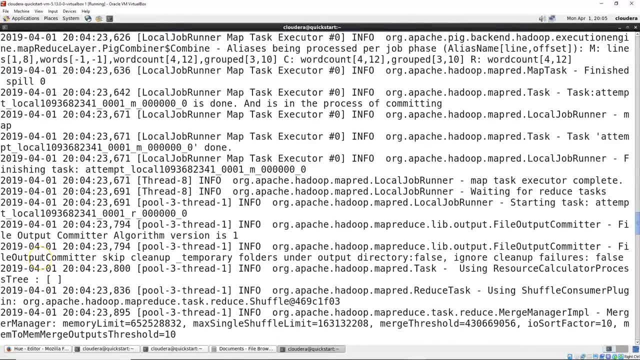 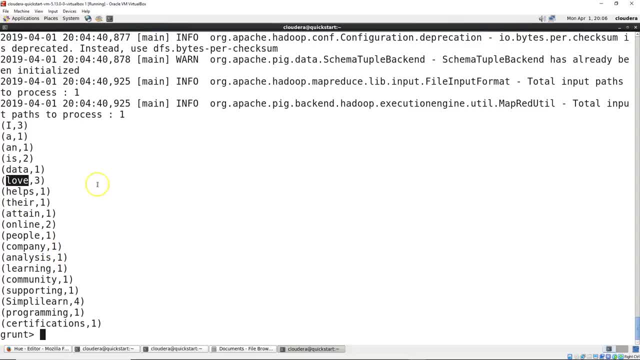 But that was the first script we put in there And then it goes through the full map- reduce, localize, run- comes out And, like I said, it's very easy to use. That's why people like Pig Latin is because it's intuitive. 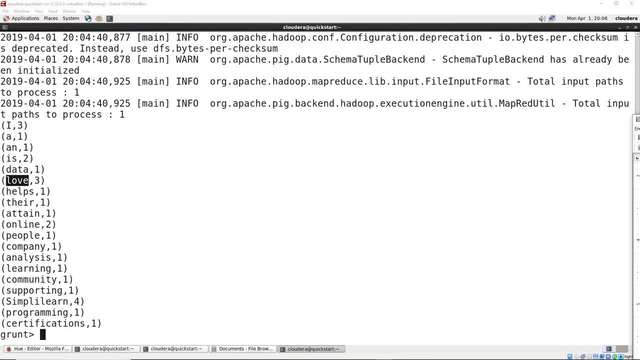 One of the things I like about Pig Latin is when I'm troubleshooting, When we're troubleshooting, a lot of times you're working with a small amount of data and you start doing one line at a time, And so I can go lines equal load. 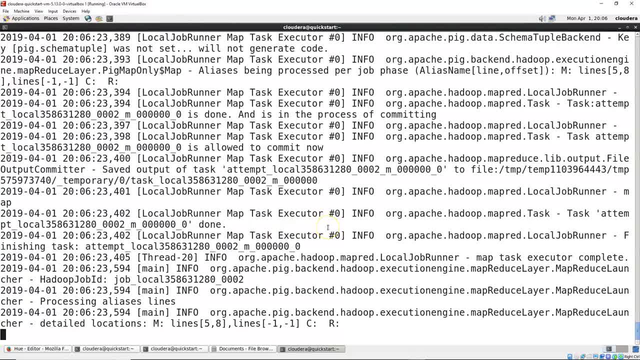 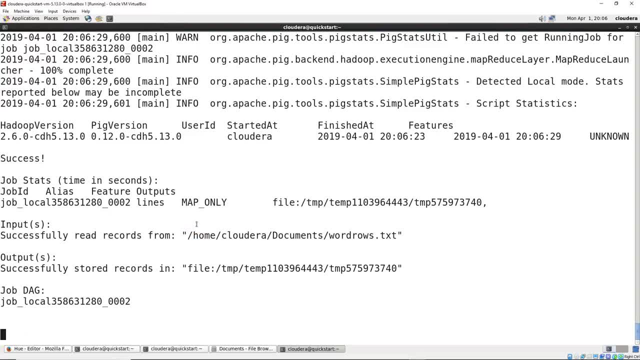 and there's my loaded text and maybe I'll just dump lines And then it's going to run running on the small amount of data And that way I can test that If I got an error on there that said, oh, this isn't working. 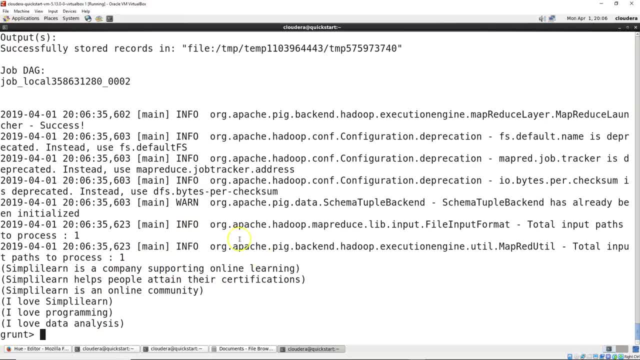 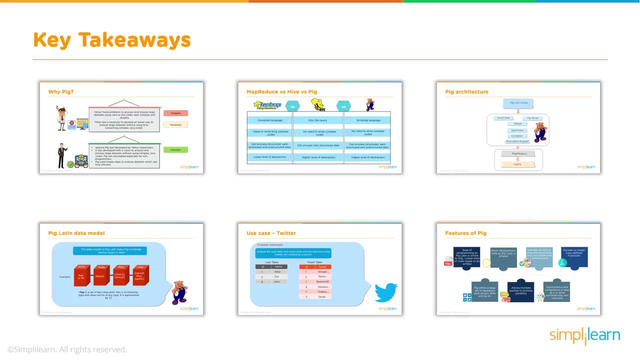 maybe it'll be. oh my gosh, I'm in map reduce or I'm in the basic grunt shell instead of the local path grunt, So maybe it'll generate an error on there. And you can see here. it just shows each of the lines going down. 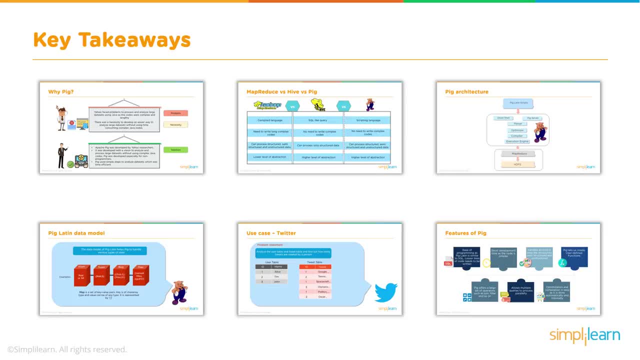 So just a quick recap. We went over some key takeaways. Why Pig? Because map reduce was very expensive in production for some of the most for running basic queries and analysis. Map reduce easy to learn. We looked at map reduce versus Hive. 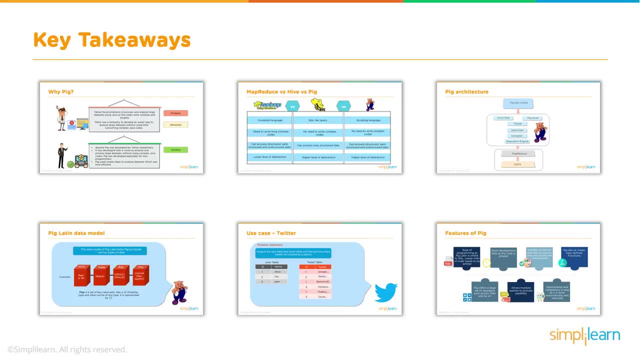 versus Pig. We found out that there's a lot of differences, like Hadoop and Hive can both partition. Hive and Pig came out because running the map reduce in Java and 80 lines of code was more than anybody really wanted to put in on a basic query. 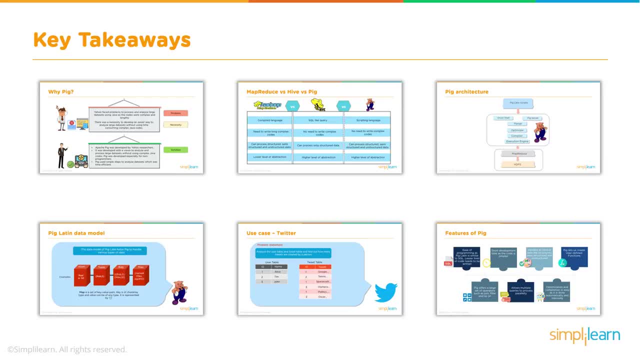 Imagine you're the shareholder and they come back and they say, yes, we can answer that question, which you need so that you can ask the next question. But it's going to take a day because our programmer has to get to the point where you can write. 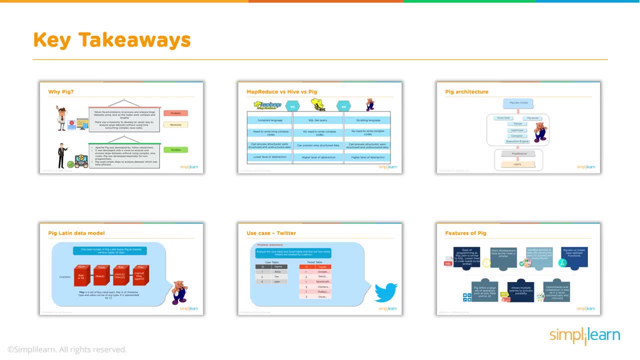 your own SQL code. You can go in there and write your own Pig Latin. We went over the Pig architecture and how that all fits together with the Grudge shell versus the Pig server. the parser, the optimizer, compiler, execution engine into map reduce.